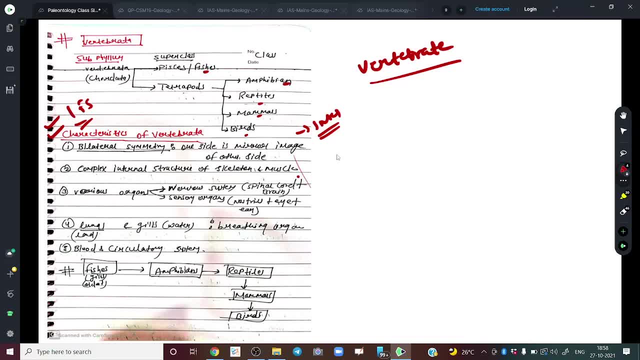 They don't have much of you know, complex internal structures. They don't have much of the skeleton or the muscle- Very simple morphology, Right. Right Also don't have much developed organs or the important life life driving these systems, like blood and circulatory systems- Right. 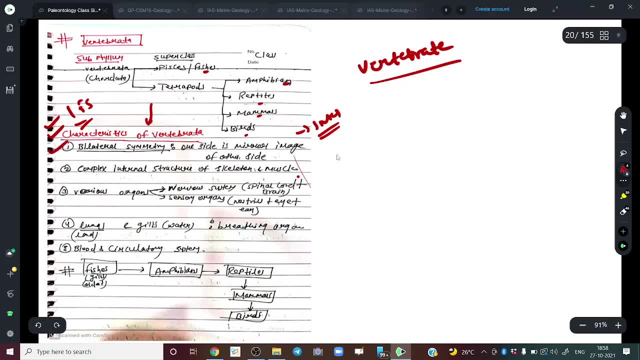 So these are the characteristics of vertebrata. What, Firstly, the vertebrates have, all the vertebrates have- bilateral symmetry, That is, the one side of there is mirror image of the other side. So a very simple thing. Like they all have complex internal structures, They have skeletons, They have muscles, Right. 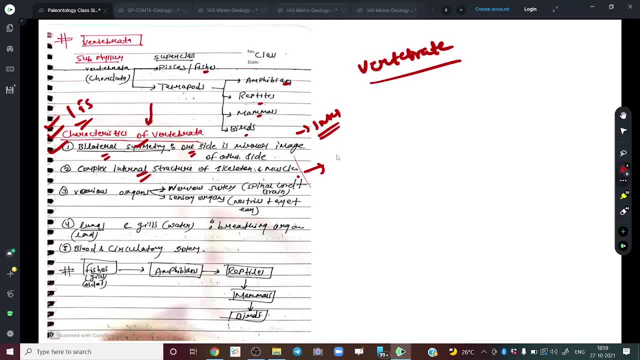 Like, And then we have bones. How many bones do we have? How many bones do we have? We humans normally have like up to 206 bones, Right. So it is a very complex system. Similarly, we have various well-defined organs, like we have, you know, brain. we have eye, ear, nose, we have spinal cord. 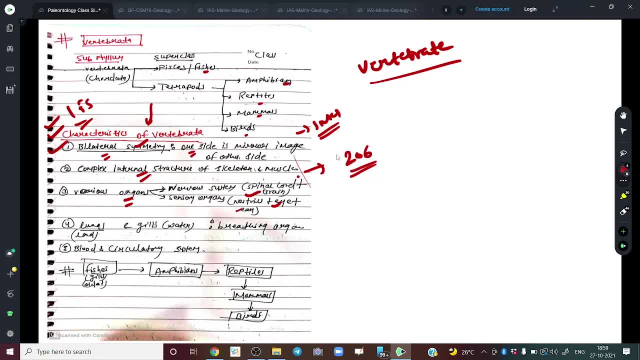 We have very well-defined organs present for specific purposes. Then we have this vertebrata. with time W W W, Some of those vertebrates is made up of large bones existing in there And therefore the sex spans. Krishna can't get many of these. 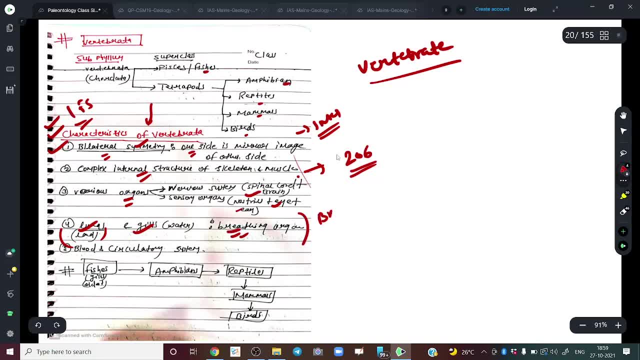 They've got a harder time getting these projetions very recording. Same thing can be done for um animals, And so they have uh bred just by turning them the nervous system right, And so it focus throughout the faisal organ that should come. look uh around that pharynx. 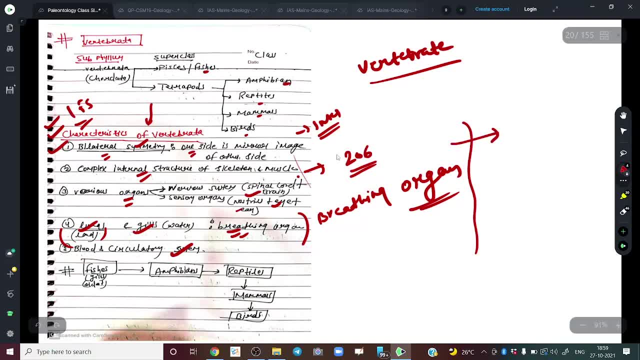 So some vertebrates develop very cross claiming f Negative, uh trunk, uh vessel, and then these vertebrates develop gills caught off guard in the examination right, and then this is also something which i think has been asked once in ifs, i think in early 2010s. so, like they asked, and this is also given in ncrt- something 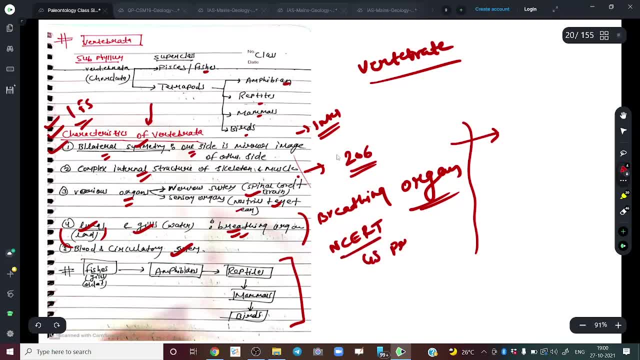 this is something which can be asked in even gs prelims, right, and something which is given in 12th geography in crt. that how life evolves, right. this we discussed in the last part. also. that the when life evolved it was. you know, it evolved from very basic cyanobacteria, right, so it was a microscopic. 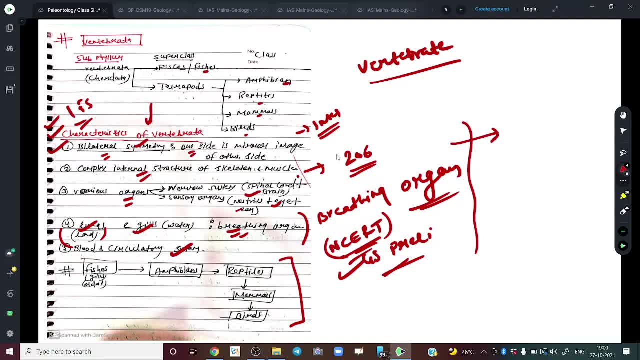 kind of a organism. then life evolved from this prokaryotes, it became new carriers. then there was, you know, multicellular organism. then, similarly, what happens? what organ development happened? some tissues, they form brain and they started, you know, developing on a particular part of the body. 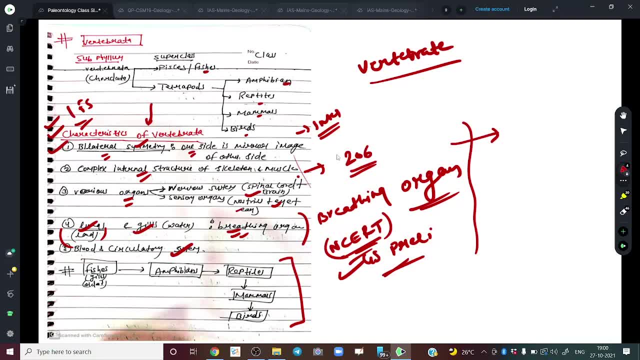 then other digestive system, circulatory system, they start started to build up lungs and gills. stronger lungs and gills just started coming up. so this is how life evolved. so in terms of phyla, or the class right, this is all vertebrata phyla also. 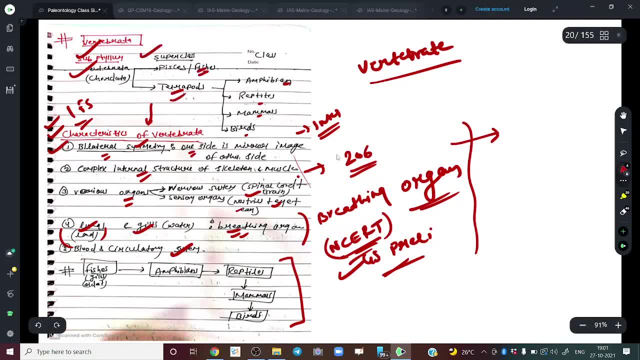 known as quadrata and classes are either fish, birth and these are the four tetrapods amphibian, these are all class reptiles, mammals and birds. so of all these, the first one is the fishes, which they evolved. they came up on the earth, so they are the oldest, they have the gills right. 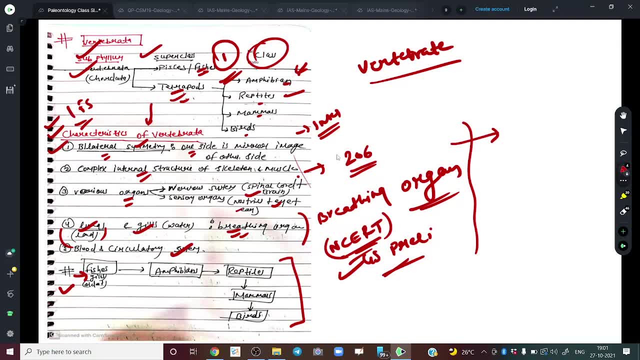 from fishes life form. slowly, gradually, they started coming from ocean to the land right, but they were flexible, they could also go back to the ocean. so they were the amphibians. right from amphibians there comes organism known as the reptiles, which could live in the water, which 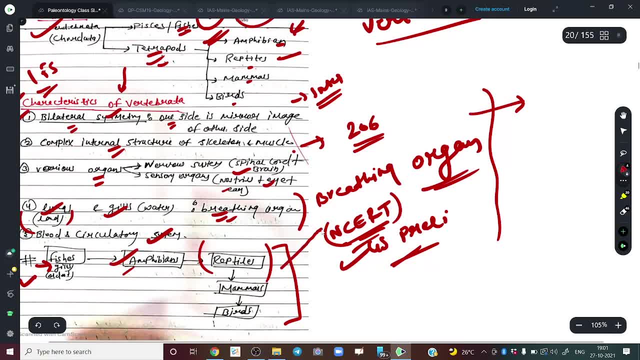 could live completely on the earth. so they were the amphibians. so they were the amphibians, the land right. So it is also not the case that first reptile came up, that only then mammals, then birds. All this evolution was taking place gradually, when even in the times, 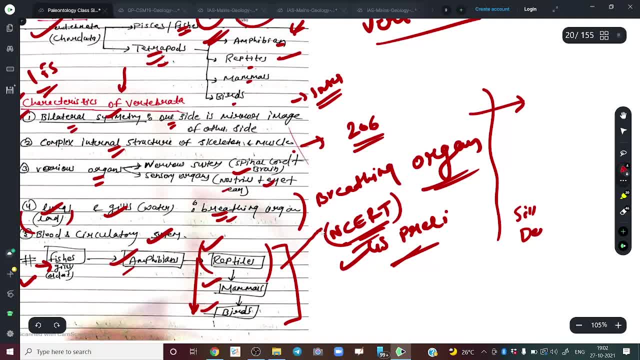 of you know the Silurian and Devonian times in geological time scale. when you know this was, we say that it is an age of fish. These were the ages age of fishes, right. Even at that time, some very primitive amphibians started to develop, right. Similarly, like 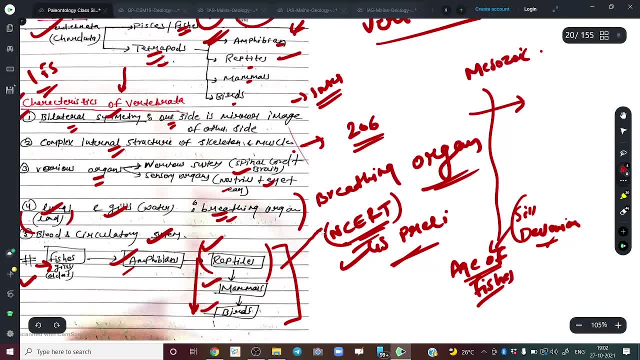 we say that Mesozoic era is the era or time of reptiles, right? So it does not mean that only reptiles inhabited planet earth. Even at that time there were some mammals, you know the first bird, Archaeopteryx. we say that it is a link between the reptile and the birds. It also came up somewhere in Mesozoic only right. Even in the Mesozoic time right, There were some mammals, also like in Cretaceous. even in Zoroastrian time there were some mammals, but they were very, very primitive and they were very, very, you can say they. 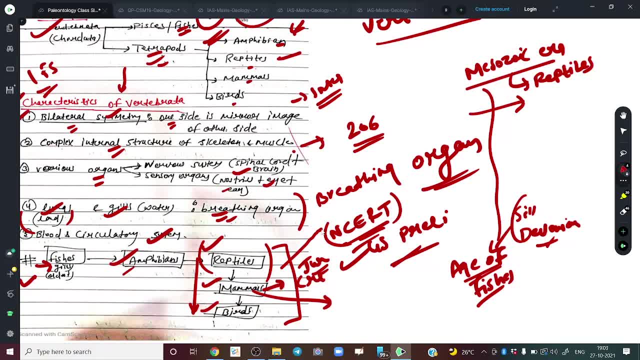 were like rodent-like mammals, right. So like those mammals, the first mammal they were, they are the ancestor of all the modern mammals. Modern mammals means human. we eat cat, dog, horse, elephant. We all have a common ancestor, and it was we all have a common 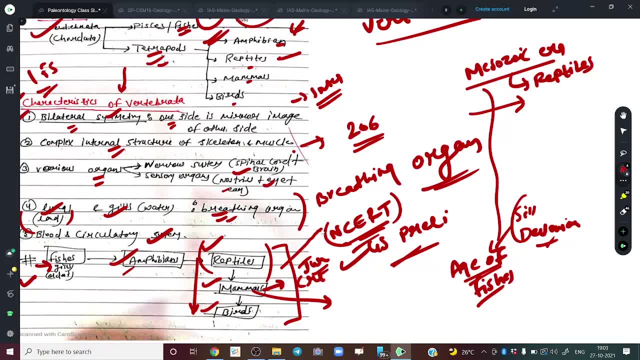 ancestor, You know, pretty much like modern rodent. It is not the modern rodent which is our ancestor, But it looked something like the modern rodent And we will discuss about this after a couple of slides. right, Why do you understand this part? So again, 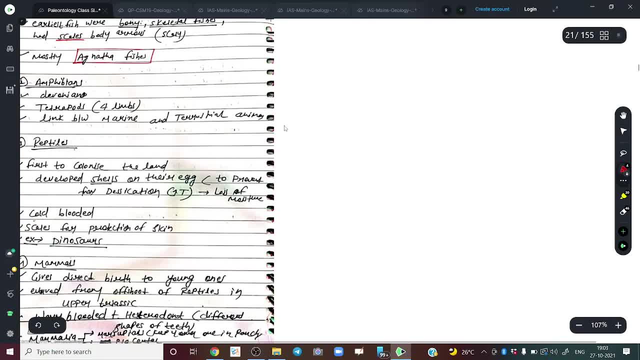 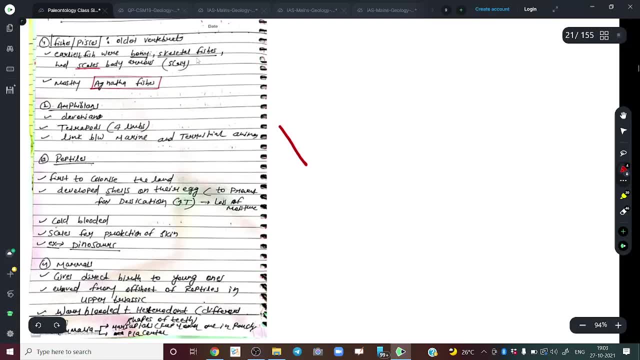 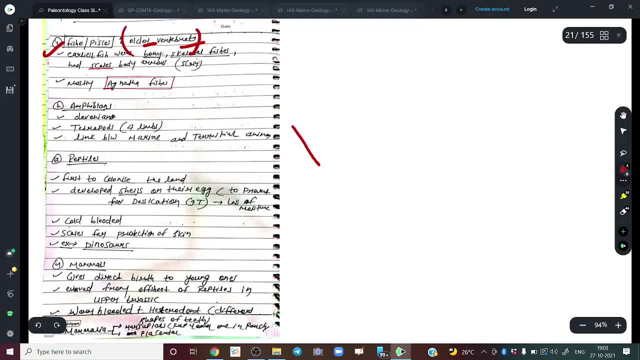 oldest vertebrates, like. forgive me for my bad handwriting, but these were just my short notes which i prepared for last minute revision, or maybe in the second layer of my notes, right, so the earliest fishes were bony. the earliest fishes were bony. they had a skeleton, uh, something like. 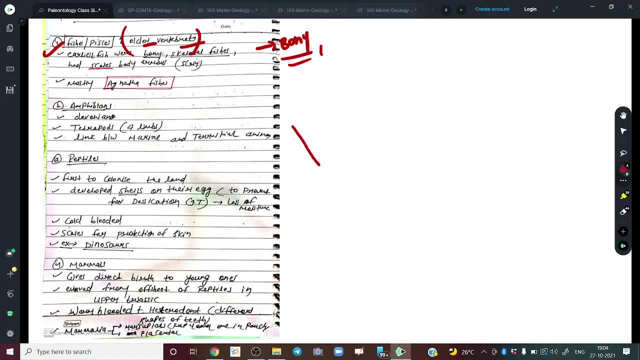 that like so uh, and then they developed. they evolved to be more adaptive to the, to be more adaptive to the surrounding right, and the earliest fishes are also known as agnatha fishes right. agnatha- this word generally means jawless, this generally means jawless right. so they were jawless fishes right then. similarly, we have the. 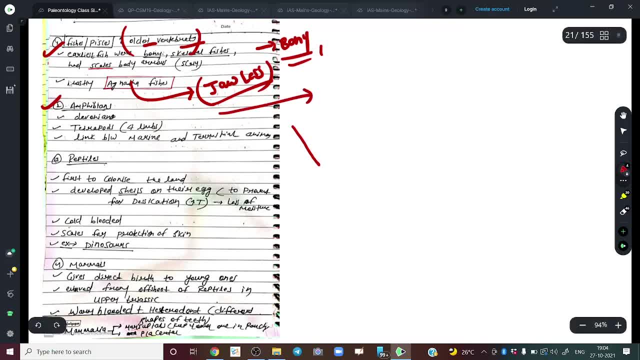 next we have amphibians, and they first appeared in the devonian time period. they first appeared in the devonian time period and we can say that they are basically the link between the marine and terrestrial animals, right, just, we discussed it. then we have reptile. they were the first to colonize the land, right? so they developed various uh adaptive mechanism to 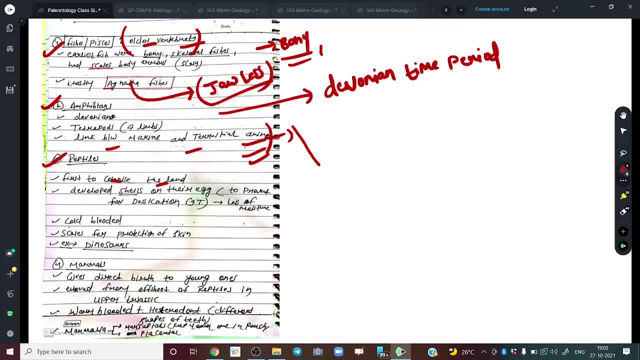 to reproduce and live on the land, like they developed shells on their egg, so which helped them to prevent the loss of moisture to desiccation, uh, to prevent the desiccation from the sun's heat. right, and we know they are cold-blooded, they have scale for protection of their skins and dinosaurs. 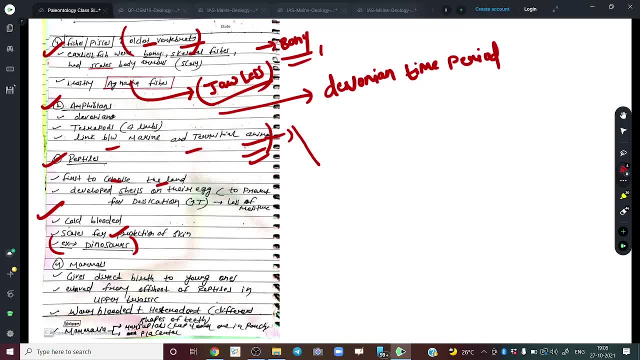 are one of the most famous example of reptiles. then we have mammals. so mammals are those animals which give birth, which give birth to their young ones, which gives direct birth to their- uh, young ones. right, so they actually evolved from an offshoot of reptiles. only in upper triassic, like in mesozoic, what we have, we have triassic. 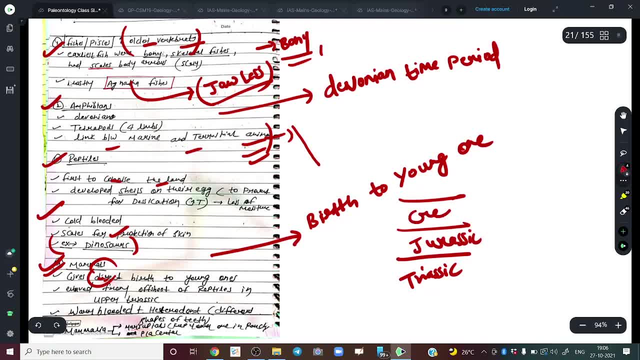 zoroastic and we have cretaceous. so it is somewhere here. mammals started not to develop. they first developed from reptiles, you know someone of the reptile only. and here we, we say that we have the first, uh, we can something we can call mammal. we. 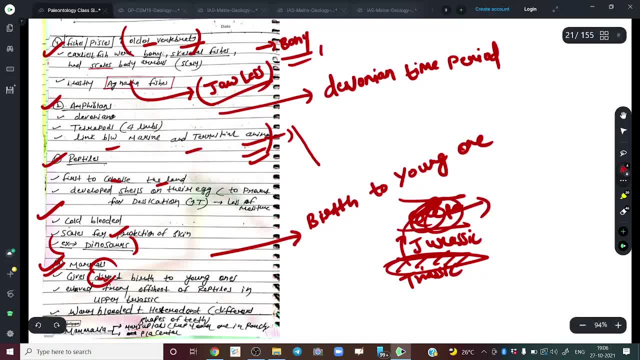 have you know somewhere? here we have the first, uh, common ancestor of mammals, right? so they are like warm-blooded, right? and and like this is just general knowledge that mammals are generally of three types. now, the most common mammals, like 98 percent of the mammals, are pleasant-born animals. like addy, hyper favs, like such a wild animal cats are Consecutor. anyone alpaca and rod viewed as very global native trying to get closer to animal nature, this kind of omnivore species or more, i am not thinking about that. then batik and other also name animal people in other countries, personality races and and orato uh, seranest. 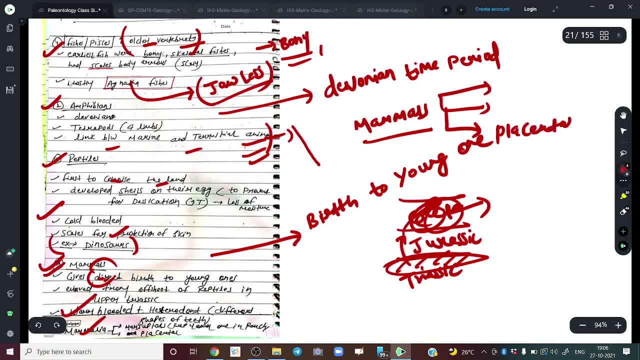 i forgot in umatch these kinds of flesh living was so i. i am very excited that it might be the most common mammal here. of the mammals are placental- like i, i know you- conceptual bees. they give birth to their young ones. they give directly, direct birth to their young ones. then we also have some as marsupials. 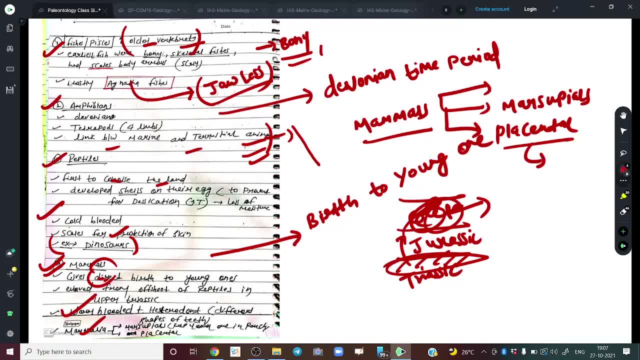 can. can you recall? where do you find these marsupials? these marsupials are those mammals which have pouch like structure where they carry their young ones like. the most famous example of them is the kangaroo. these marsupials are also found in south america. right, some marsupials are also found in 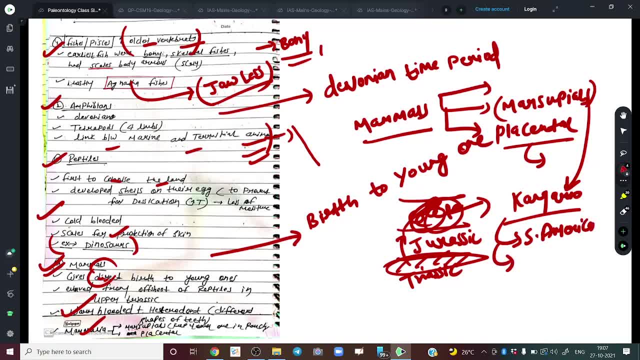 south america, but more than 95 percent of the species of these marsupials they are found in the continent of australia right. similarly, some few, very few, uh this mammals. they are also egg laying, all right egg laying mammals. so you must have heard about platypus. 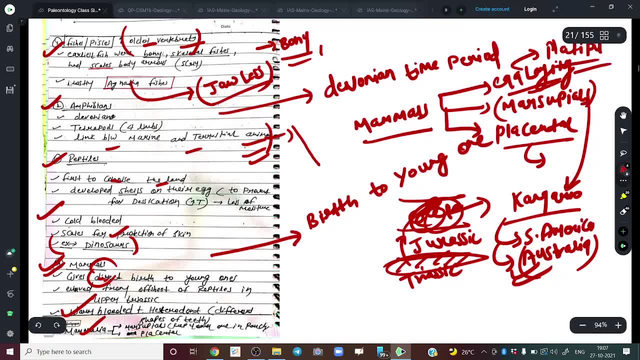 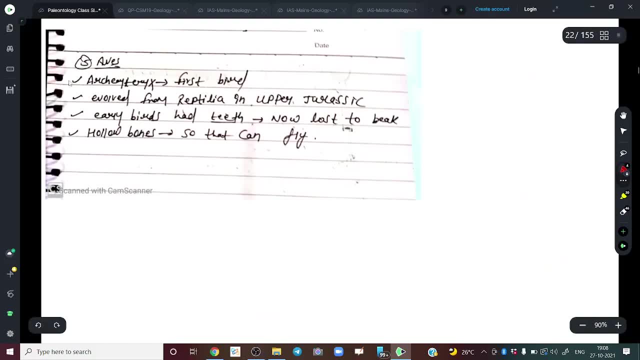 a duck-billed platypus. so it is an example of egg-laying mammals. so, in a way, actually, these are just representative of most ancient, most, you know, primitive mammals. presently most of the mammals are placental right, so this is just some very basic, and then, similarly, these are: 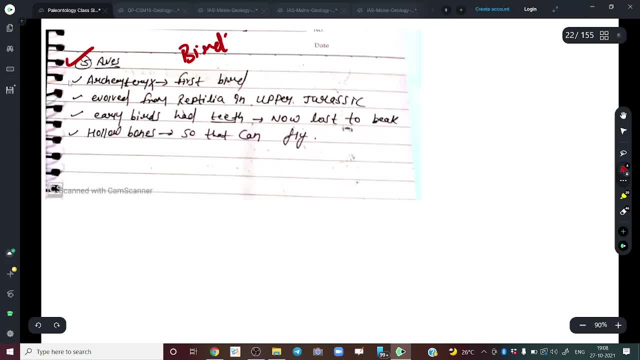 the avian species, that is, the birds. so, like the one of the first bird which we uh like call is these archaeopteryx. some books categorize this archaeopteryx as the first bird which we uh like call is these archaeopteryx. some books categorize this archaeopteryx. some books categorize this. 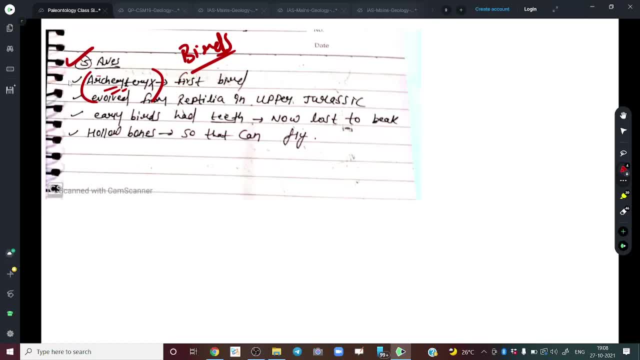 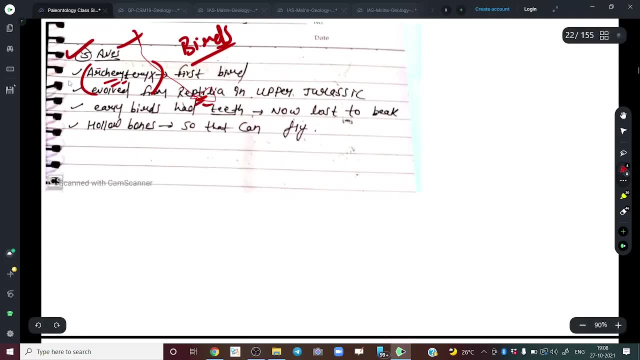 archaeopteryx. some books categorize this archaeopteryx as reptiles- right. but some books say that this is a link between the birds and the reptile right. so they, these birds, also evolved from these reptiles only in upper jurassic right and the earliest birds like they were very early. they were primitive, they were had to have a lot of adaptation, so they had even. they even had teeth right and their bones were not hollow. so they were a bit, you know, uh, they were bit heavy. but the modern birds, as we all know that they don't have teeth like their teeth is modified into. 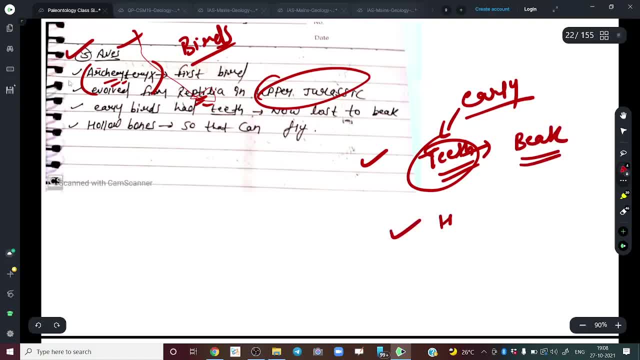 beak right and, and also their bones are hollow. you know mostly their horns. uh, bones are hollow bones, so because of this they can even fly pretty easily. so, like this was a very simplistic thing. so now this is our main topic, that is, the evolutionary trend in hominid eye. 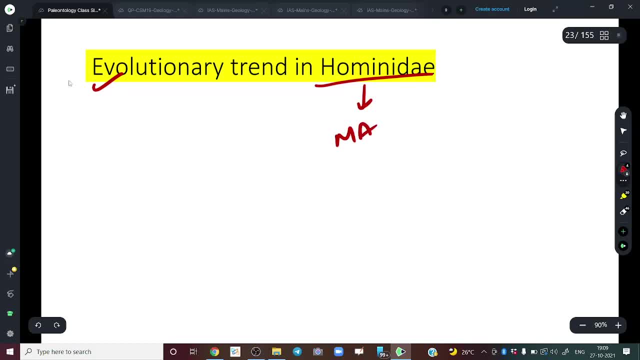 so this hominid eye is nothing but this is man. so we want to study how we humans, how this human species is, has evolved right. so we have to just trace the ancestors and we just have to understand few important characteristics and our, our topic is not just evolution, it is evolutionary trend, so we need to observe what changes are. 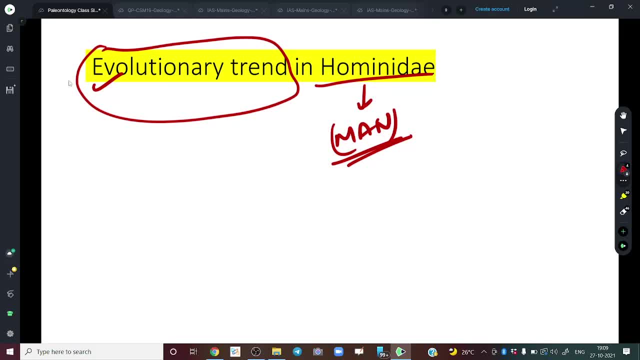 happening from our most ancient ancestor to the modern time. what changes have happened? right so, all those changes which we don't have because their social classes, they areоватьonse great. so we, about our love of space, that incredible with which we had messing an entire place über1000 years, asked for a compulsory. but no, then we want, we want one thing for our painted and enough, your do it that way. we don't have. 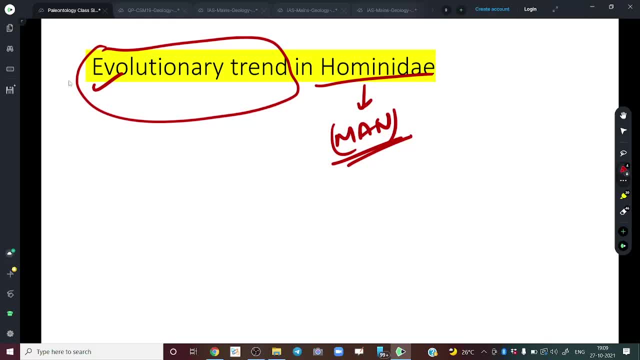 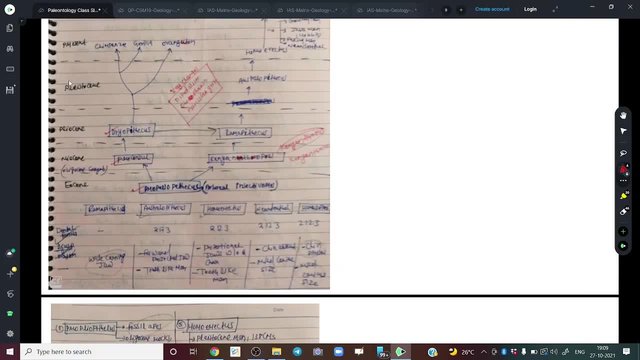 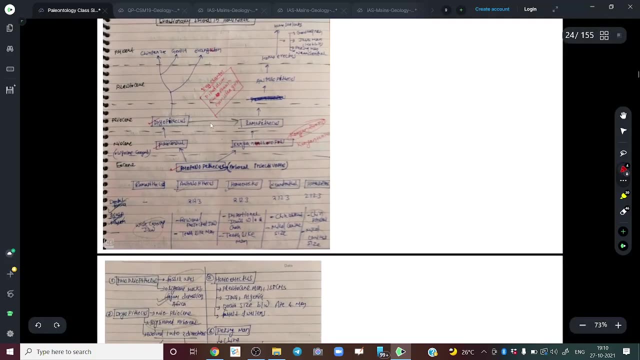 just need to remember the keywords and we need to produce all of those in our answers. so, like I have specific slide made for this, but these are my old notes, these are my old notes, so I am just giving you as a as a brief overview that ultimately we will read. we will devote at least an hour and a half for this. 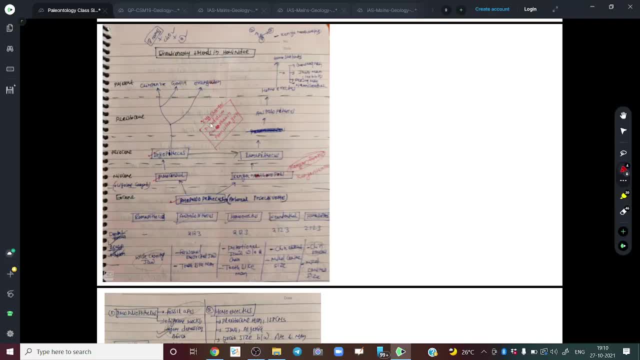 topic, but ultimately you should have a very concise notes and this evolution- evolutionary trends in hominid eye- has to be not in more than two to three pages, right like this. whatever we will read, ultimately you can put it in a diagram. this is a diagram. it's like. I'm sorry for this rough kind of a slide, but 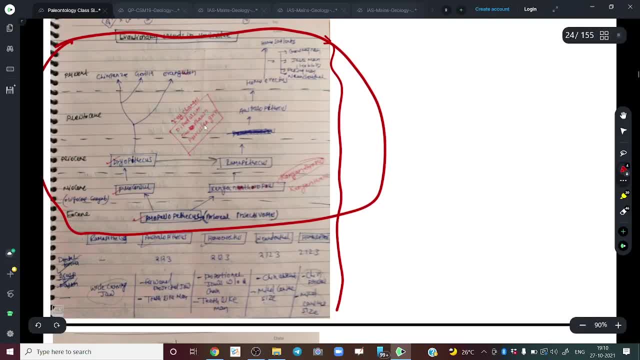 this I just want to show you. this was a rough slide of mine only I just happen to put it in the slide. so something like this: so this is homo sapiens, this is us. so what we are studying in evolutionary trends is one thing. we are studying about the name, so presently we are called homo. 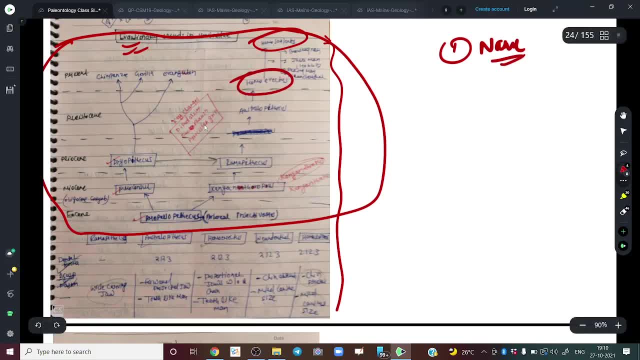 sapiens. before that, there was something which we between which is known as home or actors, like. so don't worry about this key words. we will study it so many time, you will see it so many times that you will be comfortable with this scientific name, right? so these are just ten, twelve names with you, if you remember it will. 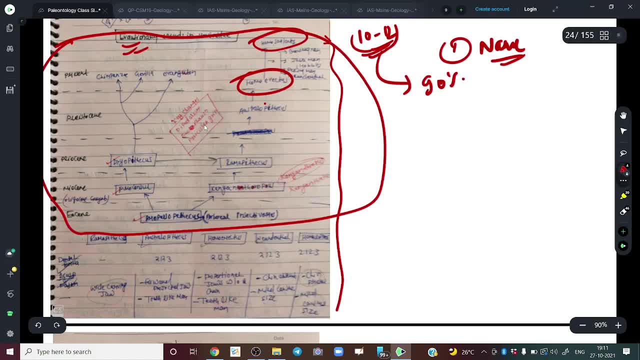 give you about 90 percent marks in this portion and this question. like we discussed in a question analysis, these are very, very, very recurrent, right, you just have to remember few basic trends which you can, you know, decipher from your general IQ itself after going through the class. and if you remember this 10-12 name, 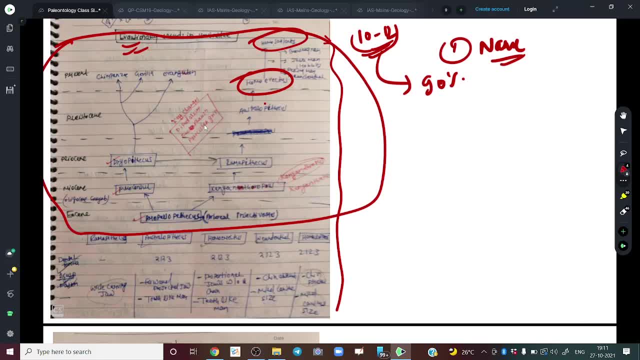 you will get almost full math. pretty much like mathematics, right? so I have also simplified it for you in this phylogenetic diagram. so we call this diagram as cladogram. cladogram is something which is more complex, but you can call it cladogram or you can call it. 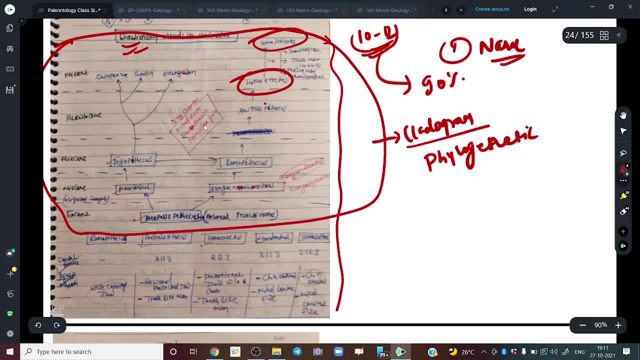 phylogenetic diagram, or you can call it evolutionary tree. okay, so just don't worry, I will go through in details of each and everything, but just to make you comfortable with few names, I am saying this: so this is homo sapiens. then we have some species like neanderthal gromagnon. it is not visible here. 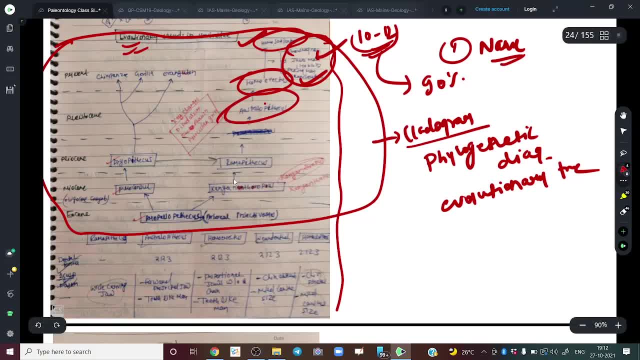 it is not visible here to bad picture, but don't worry, it will come. then we have something like australopithecus, we have something like ramapithecus canonthropus, and then we have the earliest and the oldest man-like, fossil man-like species, propylopithecus. then it has some other branches. now it branched. 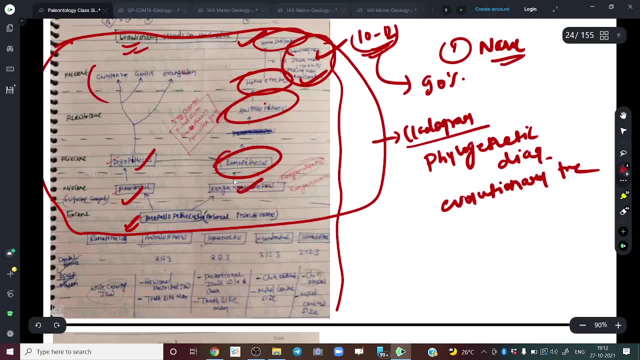 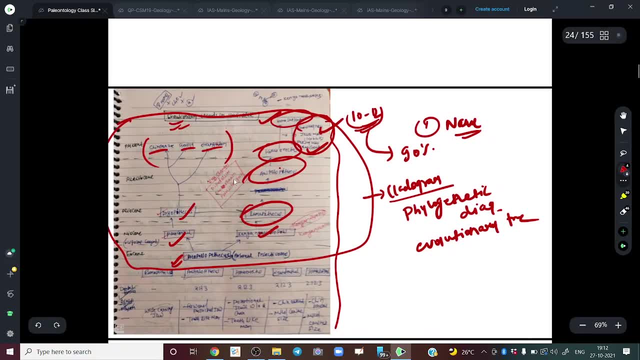 into proconsul dryopithecus. from there came the modern apes, the chimpanzees, the gorilla, the orangutans, right. so we'll see it. but this is just a sample, uh, something which we need to produce in the exam. so if there is a question on, you know, 10 marker question, you can just draw this diagram and 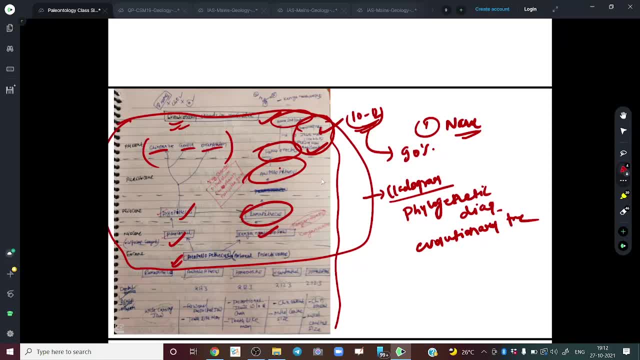 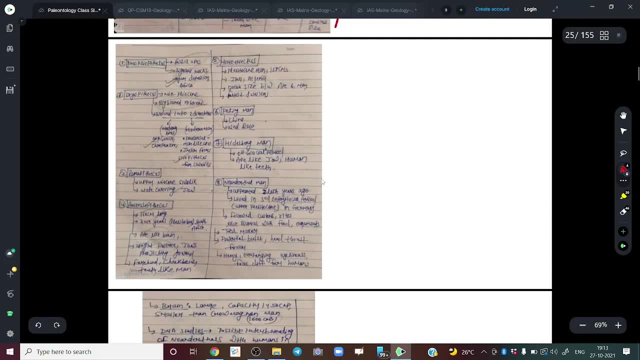 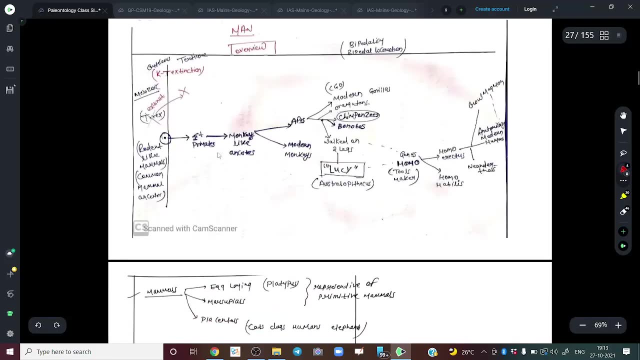 scrub cute points on it. if it is a 15 or 20 or 25 marker question in isis or is, uh right, then you just draw this diagram and just write something about all these species, which we will discuss in detail. so this is the final output. i was discussing about right, but 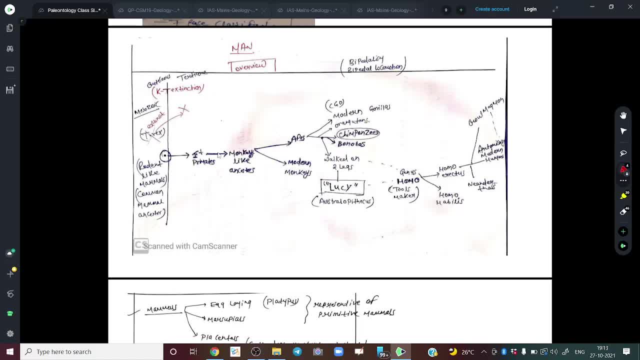 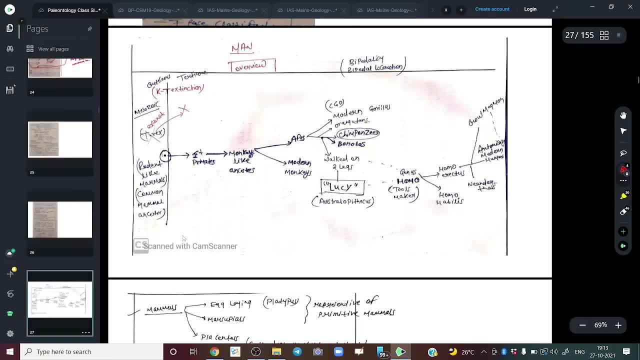 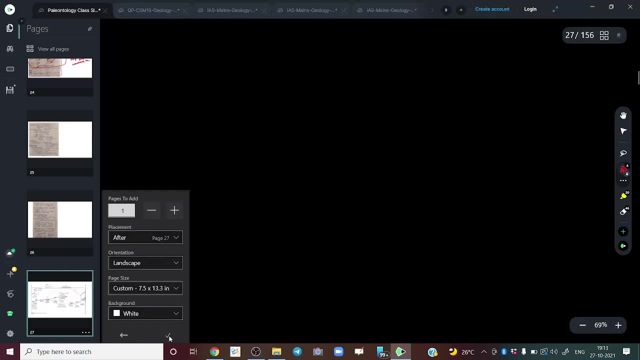 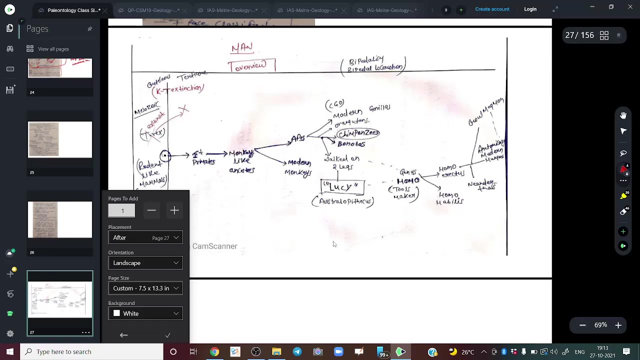 don't worry, we are yet to start the topic. so, like, just to explain you, i'll i'll just firstly i'll share what actually is happening, right? so? so okay, we now we will just go through what actually the scenario is. what are the conditions in which this evolution is happening, right? so we'll, we'll write it here, so like we can trace. 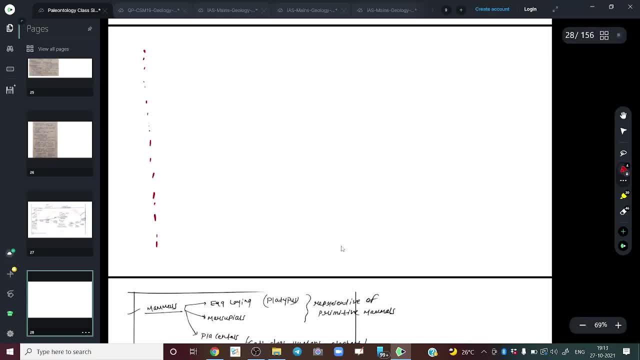 we'll trace this evolution of humans from this kt boundary. what is kt boundary, like kt is actually? this is cretaceous time period, right, and this is tertiary right. so this is mesozoic era and this is cenozoic era. so, at the boundary of mesozoic and cenozoic, 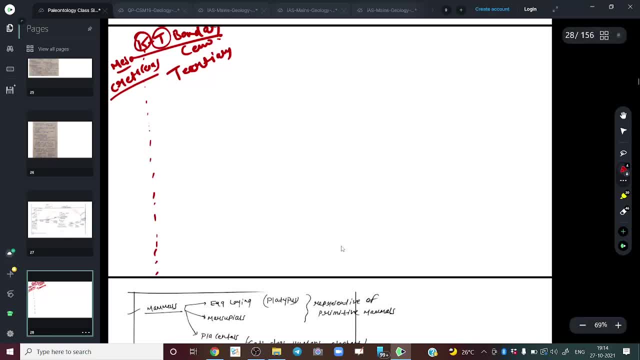 what happened? you must be aware that there was a mass extinction. there was a mass extinction about like more than 70 percent of the species on the planet earth. they got extinct, they got disappear forever, right, so this nosozoic era was the era of reptiles. other species were also there, but it was the mighty dinosaurs which dominated the planet, the earth, till this time, in the Mesozoic era. right, the species like you must have heard about t-rex, the mighty t-rex it. it used to inhabit the planet earth in this time, but what happened is this: 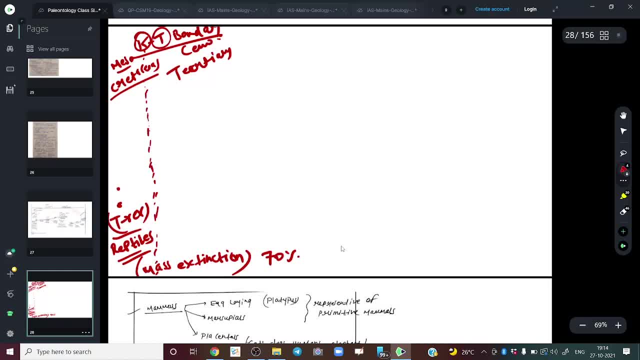 boundary is due to whatever reasons that we'll discuss, so that is not important in this context. so there was a mass extinction and what happens is that this t-rex got vanished at this boundary. right along with these t-rex there were, there were some mammals, right like we discussed. so there were some very primitive rodent like rodent, like mammals, right, mammals. so you, you can say these, these most primitive rodent like mammals. they were there in Cretaceous, but they also happened to live in the Cenozoic time, also, like they didn't go extinct. a lot of other mammals, a lot of other, you know, species. they did go extinct, but this most primitive rodent like mammal, they happened to survive this mass extinction period right. so, from this rodent like mammal, the common, which we can call as the common ancestor, right what evolved. 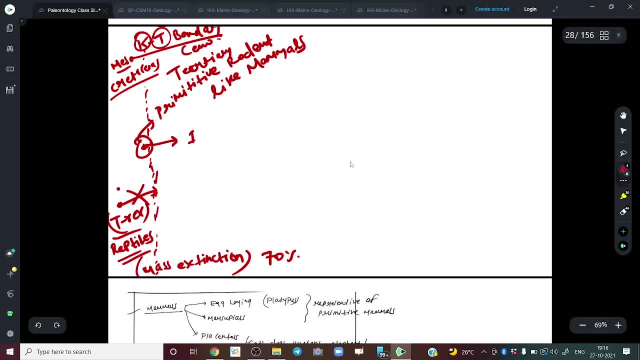 evolved were the first primates, like somebody asked in class. and what are primates? primates are what primates are, basically a monkey like creature. right, if you, if you have to give some example of modern primates like like monkey, would be an example for that. like monkey like ancestors, they're pretty much. like modern monkeys, but like they are not actually the modern monkeys, like modern monkeys also evolved from these primates only. but all right, so from this first primate what we have is we have this monkey like, we have the first monkey like ancestor, like they are even more primitive, but then from here we have this monkey like 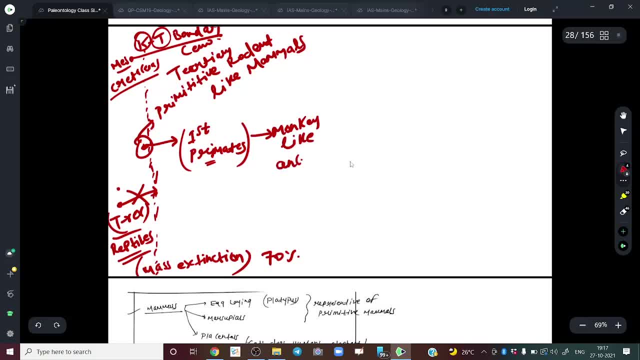 like ancestor, and from the, from these monkey, like ancestors. we have what we have. we there was a lineage towards apes, the modern apes, and we have the lineage towards the modern monkeys. so what are the example of modern, modern apes? Can you recall name of few modern apes? 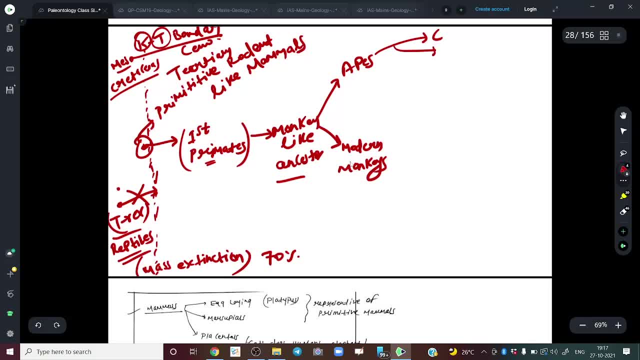 Like I say that we have C, G and we have you know O. We also have something we call it bonobos. If you have, if you know about it, these are right. So we have bonobos. 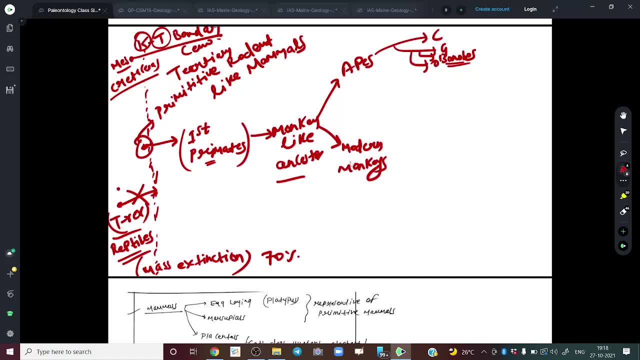 So CGO is what C is for chimpanzees, G is for gorillas, right So, and O is for orangutan, right So from apes we have this bonobos, From here, only actually these chimpanzees. let me draw it even in a more clear manner. 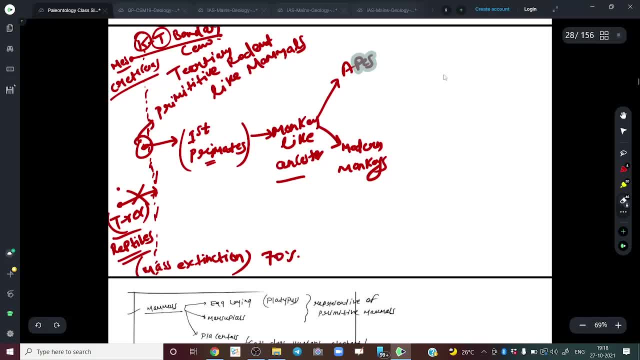 Right. So it is something like This: From apes, we have, from apes, we have the modern gorillas. right, we have modern gorillas. From here, it says there was a branching, and from one of the branch we have orangutan. and from here we have what chimpanzees. 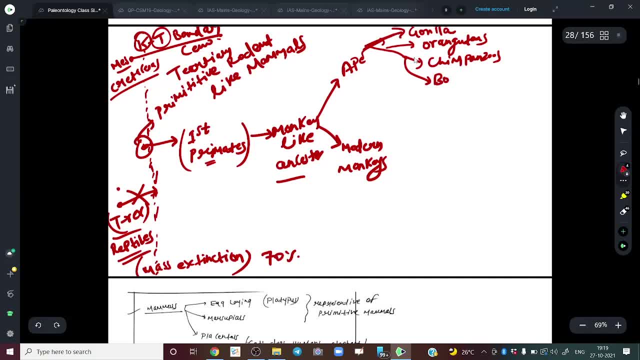 And this is also we have. we have what we have, bonobos Like- if you will see the genetic studies- the most genetically closer species on earth to humans. these are these two chimpanzees and bonobos. 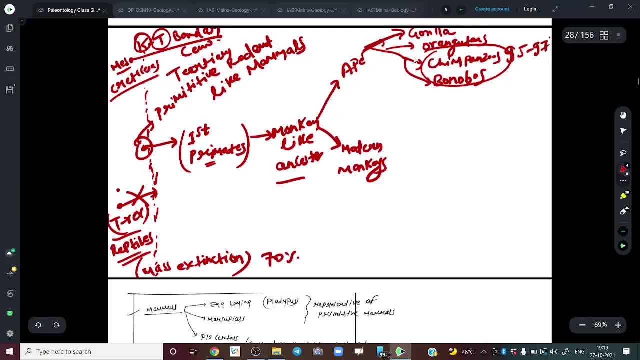 We have about 95 to 97% DNA similarities with these two species. right This bonobos. this is very rare. This is found in just maybe a couple of forests of Africa. Right? So like this is it. 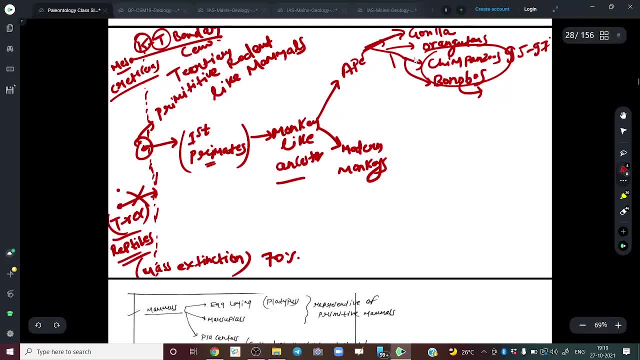 Like, what major thing happened is from here only another species evolved, And this is what is important. right From here only there is evolution. of what? evolution? of a species which could walk on two legs. Now, we still are not very sure about this particular aspect. 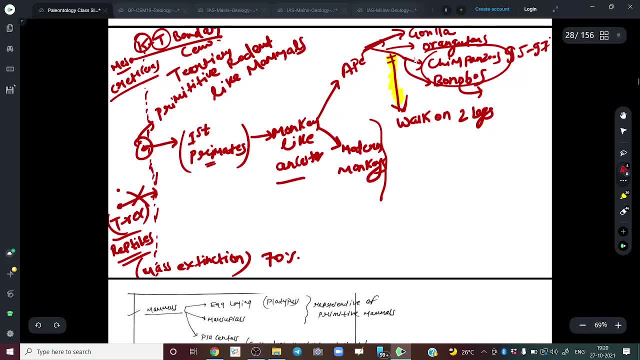 But we did found some, you know- fossil a few years ago in some parts of Africa, in the Ethiopian region of Africa, And it is very famously known as Lucy, the Lucy fossil right. It was actually a fossil of a female right. 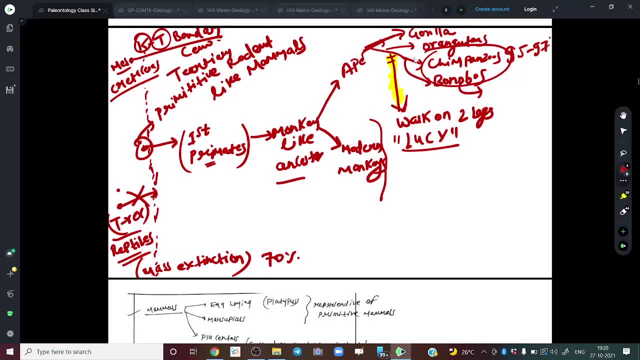 And there were almost conclusive proof that this species could almost walk on two legs right. So like walking on two legs, this phenomena is known. It is known as bipedalism right. So this species was bipedalism. 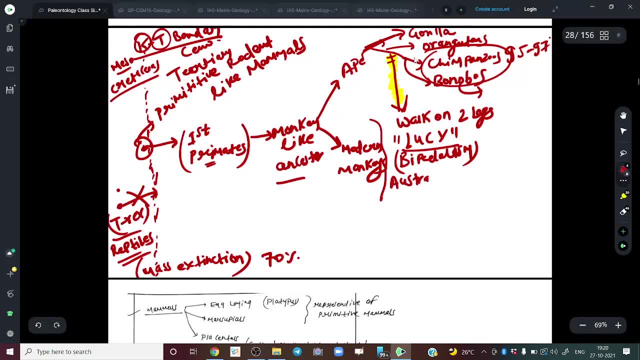 So scientifically they call this as Australopithecus. So we can say that from apes only we have first ape man And we call it Australopithecus. In some text you could also find this as Australopithecus. 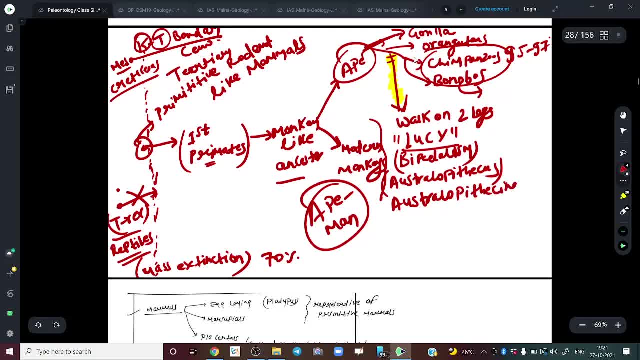 Astralopithecus, But you just want to solve this in real life. There's nothing the answer for that, that we cannot find any more, So you can have. this becomes the Delia podium. I'll tell you that. if you want to know, you can add questions in the comments, right? 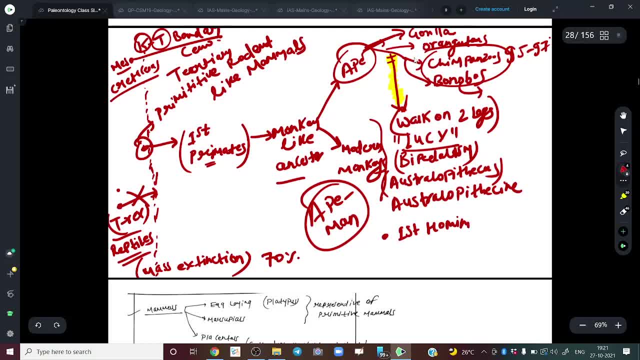 Next, you can see the recipes directly or you can link 20 persons If you would like to know the details. so we have shared this with our guests, right? No, this guys. so I would like to explain you this in this video. Let's try to find it. 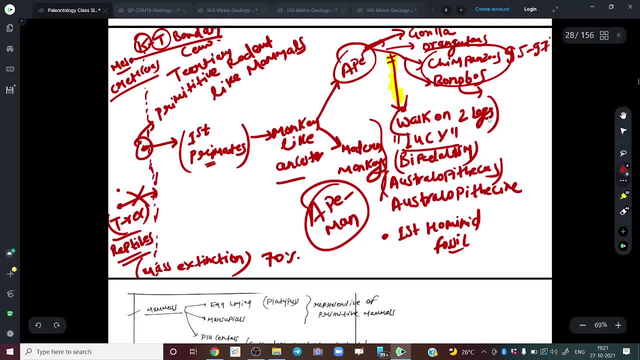 so what? what? what I happen from this? like there is it all right. so from here, what happens is from this australopithecus, sorry, from this australopithecus, australopithecus. what happens is there emerged a new genus, which, which is known. 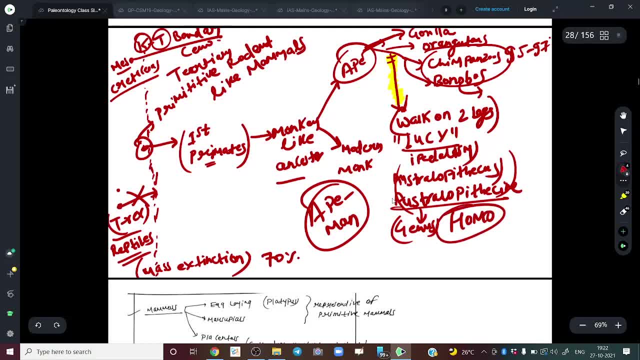 as homo. like the genus homo, it evolved from this australopithecus. so the importance of homo were they were bipedal, plus they could make tool, so they are known as tool makers. right tool makers means they work, since they were bipedal. 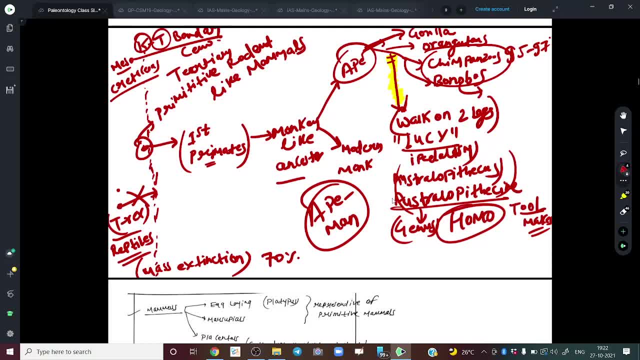 they had. they have their hands free to do all kind of bra path, like they could make this, what we call it. they could make spear, they could make, you know, weapons, sharp weapons, which they can use to kill animal and, you know, increase the availability of calories, meat right. it's time they also control fire using their 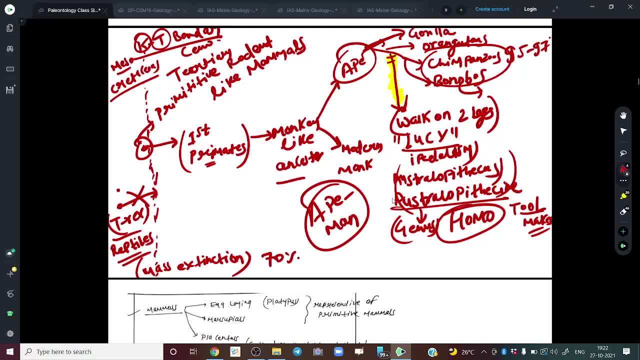 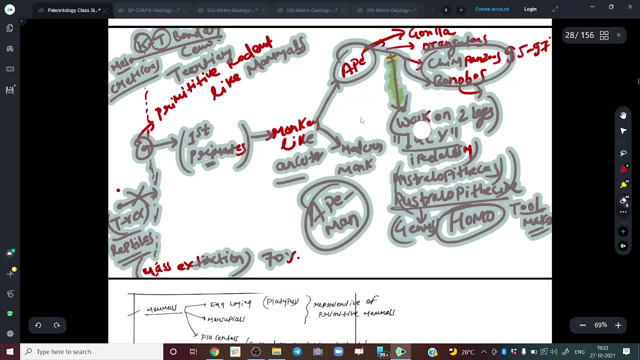 hands. so this is like the evolution start. so from here, like, let me make it a bit more, I'll rub it, I'll make it a bit more, I'll rub it again, the for your revision, and then we will preserve my, then we will preserve my you. 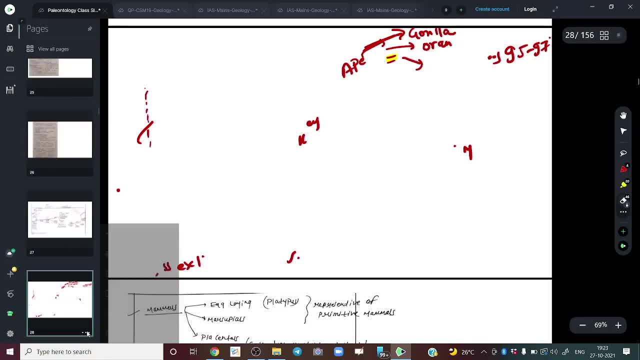 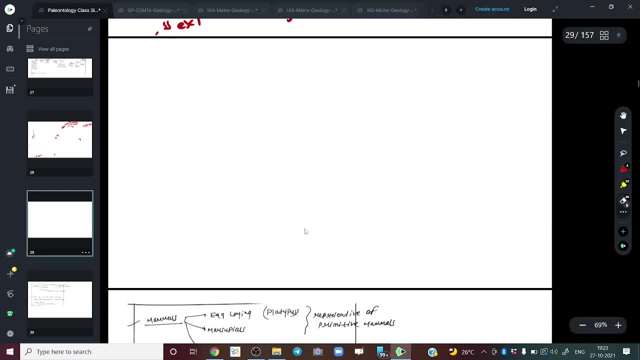 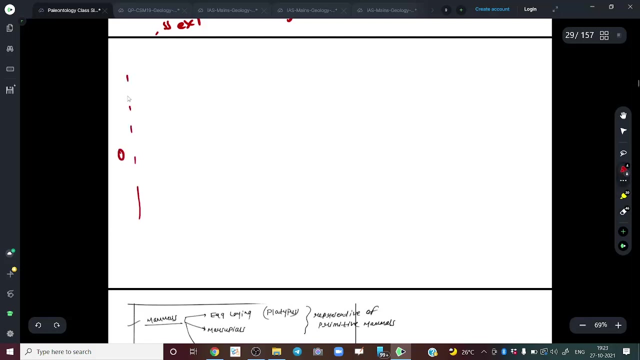 better we will use a new thing, better we will use a new thing. right so, right so, right. so What we have till now We have in this Cretaceous Tertiary time, we have a very rodent-like ancestor. right, We have a rodent-like ancestor. 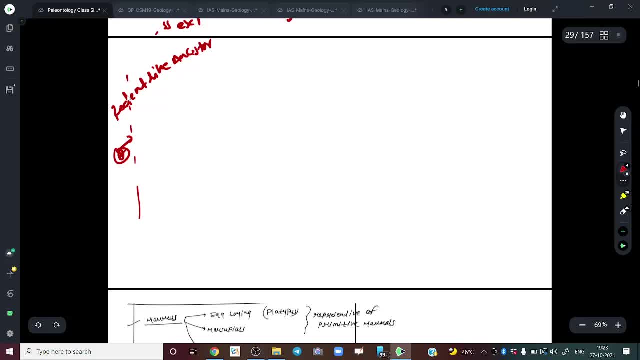 This we can say as the common ancestor, common ancestor of mammals, of all the mammals. right From here evolved the first primates. From primates evolved the monkey-like ancestors. right, They are not modern monkey, but they were monkey-like ancestors- and from them evolved the modern primates. 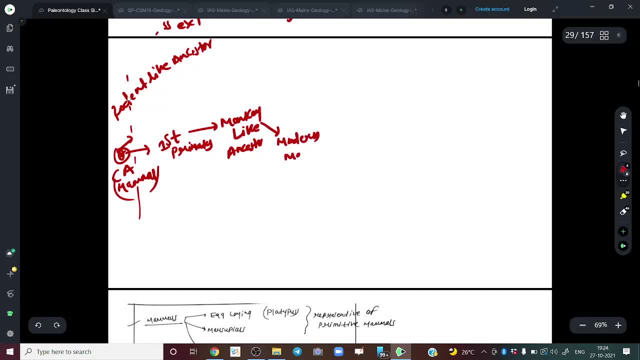 From here also evolved in a different lineage. What evolved, Evolved, were apes, right. So apes, we have the gorillas, the modern gorillas we have. you know what we have? We have chimpanzees. 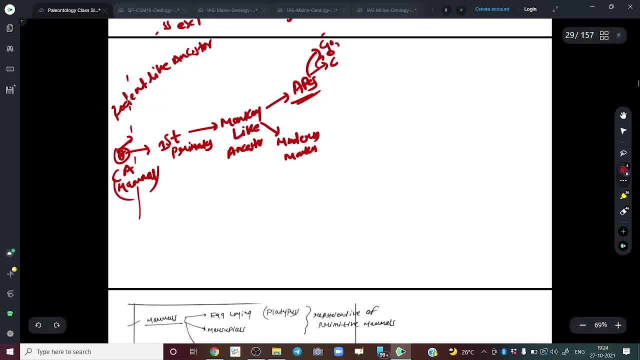 we have orangutans, right, So we have gorilla, we have orangutan, we have chimpanzees and we also have bonobos, And from here only they are developed. what The Lucy? the Lucy fossil species, right, So we call it Australopithecus. 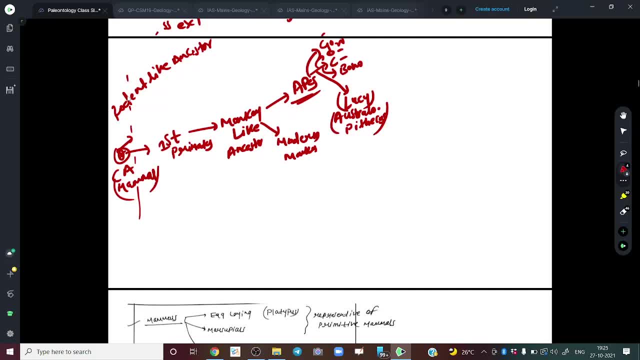 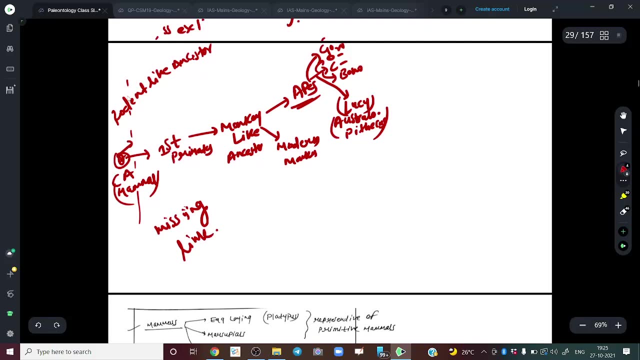 It is also known as Australopithecine. So what is its significance? It is basically a link between the apes and the modern humans. It is sometimes termed as the missing link, So it can be used for many different reasons. 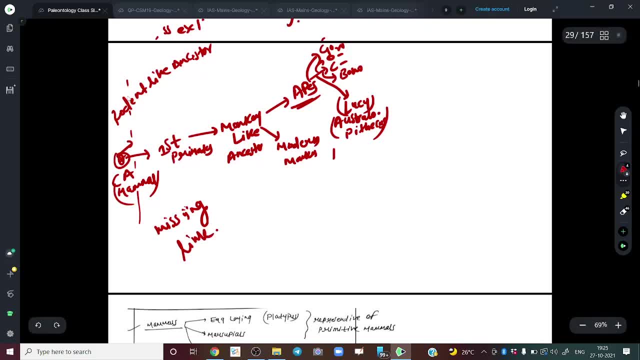 Right. so their significance was they started to develop bipedalism. they could walk on two legs, right And from here we say that from Lucy or from Australopithecus, or from some of the ancestors of Australopithecus: develop right, develop what, Develop the. 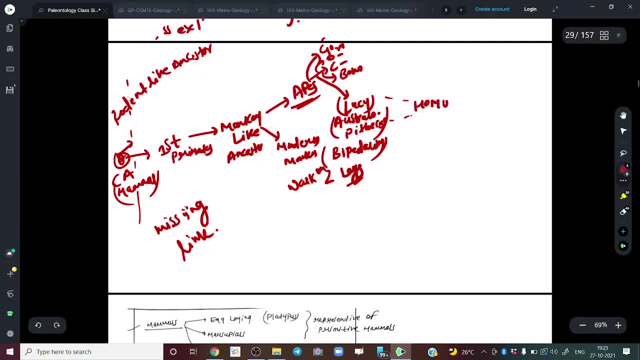 what developed the genus Homo. so we have Homo's here, so they are known as tool maker. tool is related to basically the weaponry which could be used in the forest: using stone, using wood, all these things from Homo, this genus evolved. there went various lineages. 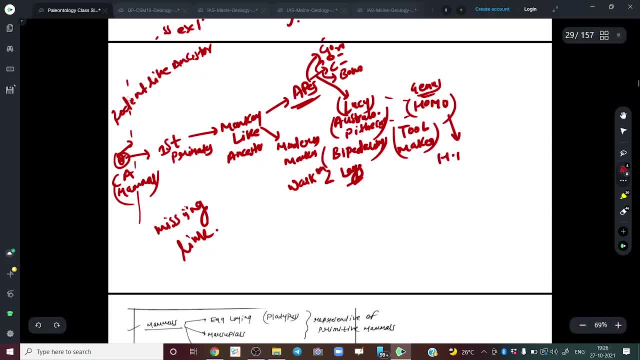 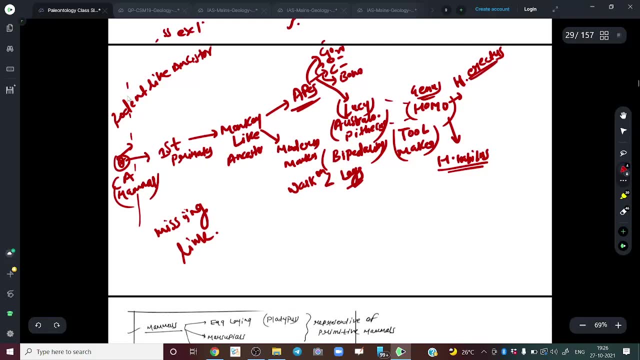 like one of the tree. it goes to Homo habilis. then it also goes to something we call as Homo erectus. so they were completely erect, they were completely bipedal and their spinal cord was completely erect and from Homo erectus developed, which what we call is anatomically. 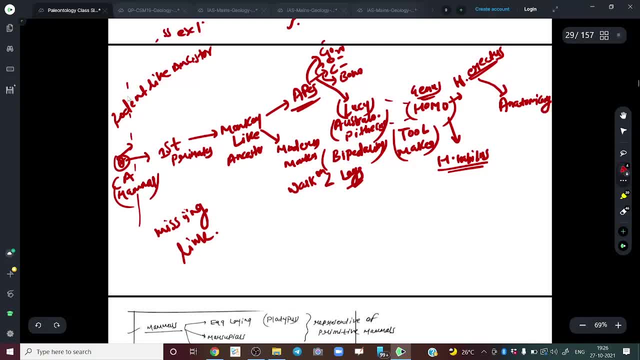 modern humans. I hope it is clear till now right? so like this is the basically the evolutionary. this is an overview of what actually is happening. so evolution is bit more complicated. there are more web going through, there are more species. some species are not even known today. 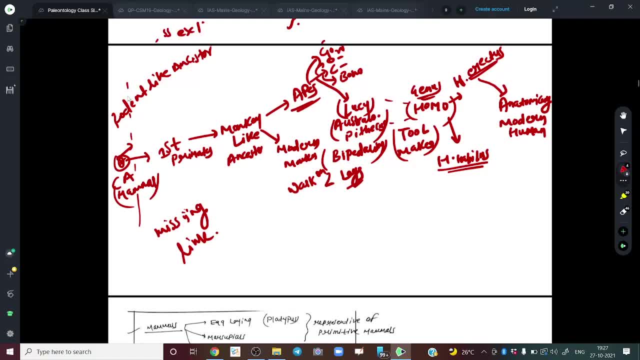 but this is something which we can write in exam, More or less a complete picture of what was actually happening, obviously from Homo erectus. there are some debates. some says that not long ago, just, you know, 30 to 50 thousand years ago from now on, we have some other species of humans also right, so like we, 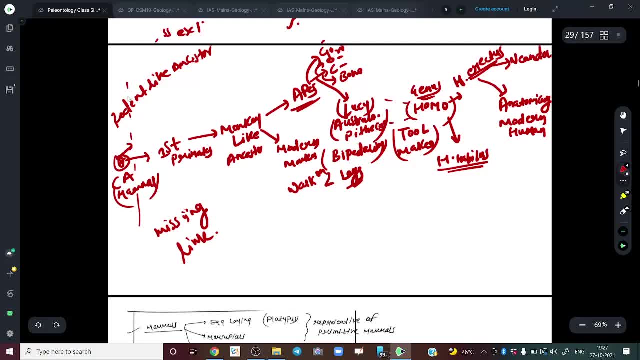 talked about Neanderthals. you must have heard about them, maybe Neanderthals. so these species, or these human species, they were found in the Neanderthal Right, In the valley of the Germany right. similarly, we have some other, we have, you know, Cro-Magnon. 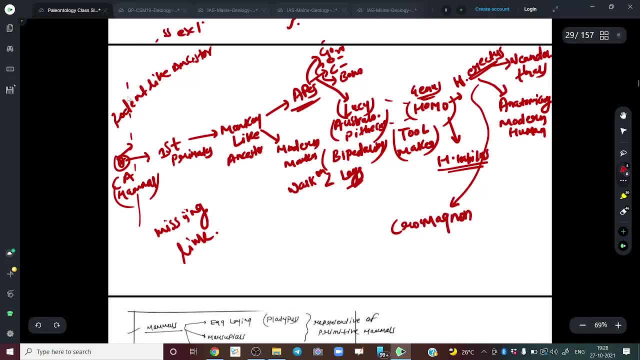 you know, this is found in the Cro-Magnon, that is, in the France, right. we have some other also. we have Java man- it was discovered in Java. we have Peking man, discovered somewhere near in Peking, right. so we have this. so, okay, this is something which, so I hope you. 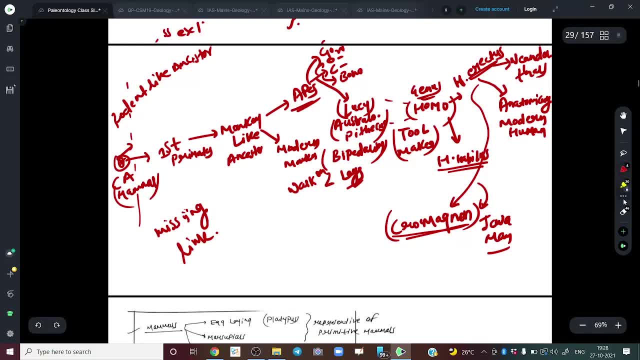 understand what is actually happening. so like just as an overview, right. so we have this first mammal, rodent-like mammal. it could be termed as common ancestor of all the mammals. from this evolved the first primates like the monkey-like looking earliest ancestors. 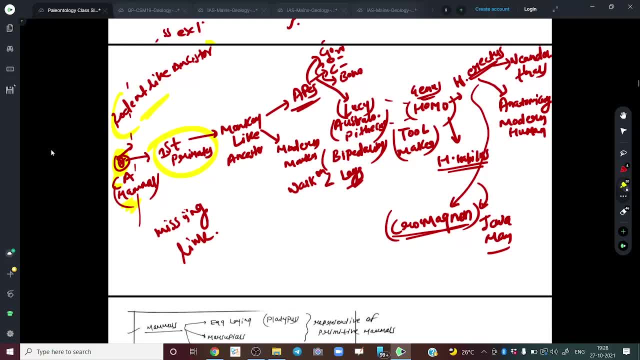 of ours, so we call them primates, from primates developed like monkey-like ancestor. from this monkey-like ancestor developed the modern monkeys, right. so you must have seen the modern monkeys right, And from here a different kind of primates, right. so we have the first primates, the 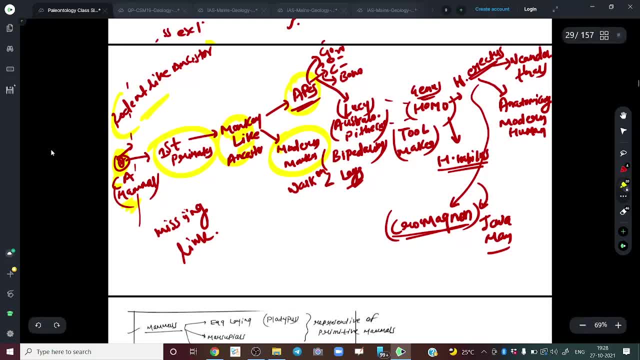 modern monkeys. right, so we have the first primates. right, so we have the first primates from this Apes. this is a different lineage. it developed to Apes. so you can see this, modern monkeys, these are not our ancestors, right? this is a different branch, our lineage. 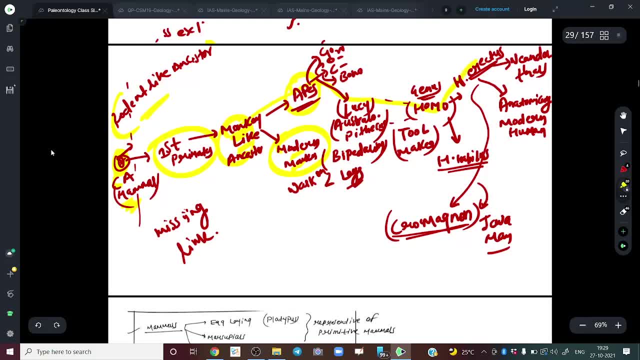 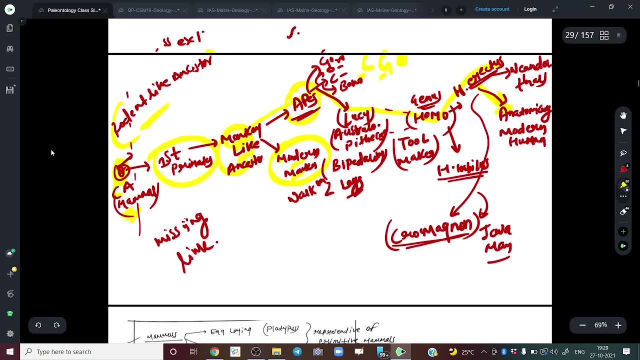 is coming this way, right, which way Homo erectus say. and then here this is our lineage coming. so these modern monkeys, they are not our ancestors, right? so from this Apes developed PGO, CGO. C is for chimpanzees, G is for gorillas, orangutans and also the. 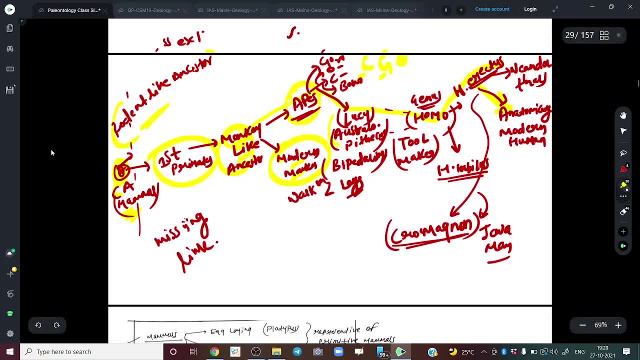 bonobos, And from here developed the first species which could walk on its two legs, the bipedal locomotion, and we call it Australopithecus. From Australopithecus developed the most important homogenous: we have Homo habilis and Homo erectus, and from Homo erectus we have anatomically modern humans. So there was a question in the class that said: why do we call them anatomically modern humans? We call them anatomically modern because DNA wise they look like us. the anatomy is pretty similar In them and in modern humans. there is not much difference, DNA wise. 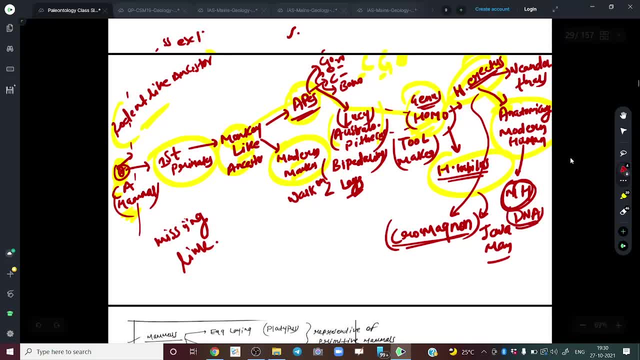 The anatomy is almost similar, But what is difference is the culture. They might not be as sophisticated as modern humans In terms of language, in terms of cultural aspects. So this is something which is in terms of economic, in terms of the way they live in all these things. 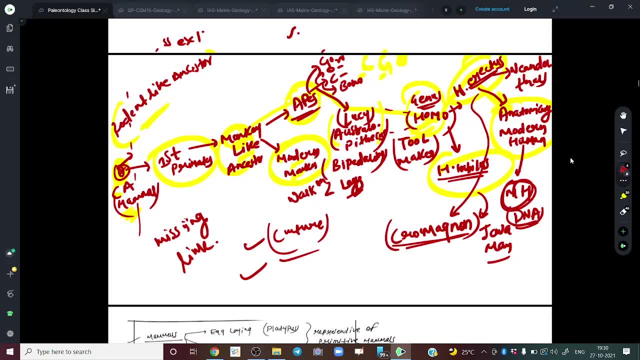 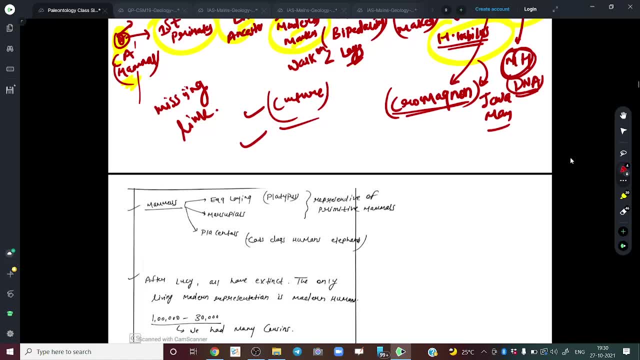 So this is the difference. Cultural differences are there. So that is out. So this is something in full overview And now we will just go through in detail of this and that's it. That will be. we will be done with this topic. 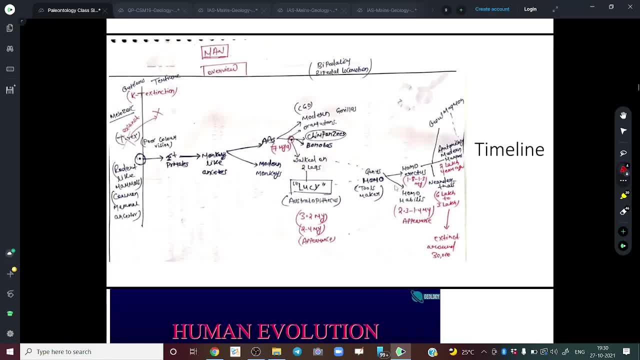 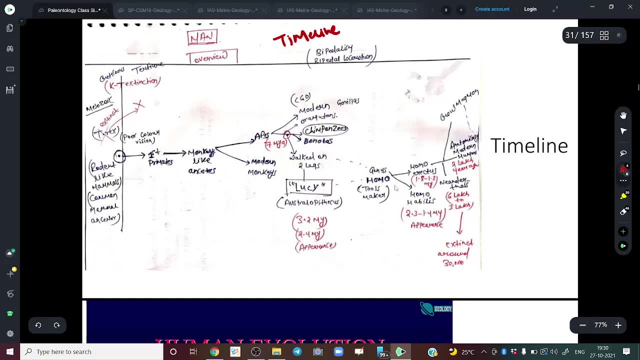 So, like this is again a slide Here, I just want to give you an overview, Your timeline. If you are interested, you can also jot down the timeline That when all this is happening. So this first ape, Like first ape, like species, it occurred somewhere around just 7 million years ago from today. 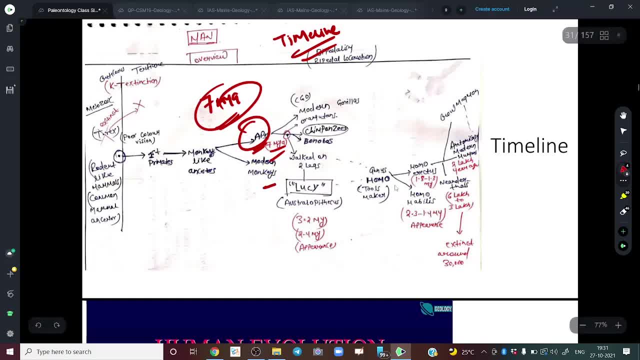 Right. So this is the ape, This Lucy we talk about. when we dated its age it came out Like there is still not complete, you know, complete understanding between the scientists About the real age. Some say that it is somewhere around 3.2 million. 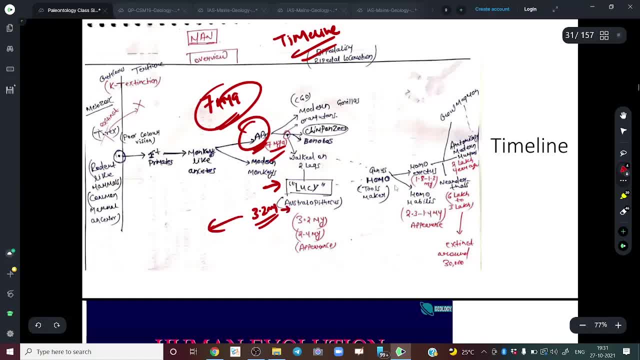 Some say that it is older, Some say that it is younger. So, like you can write it, 2 to 4 million years ago- Right, Even you can write 3 or 2 million years ago- appeared the first species which could walk on its two legs. 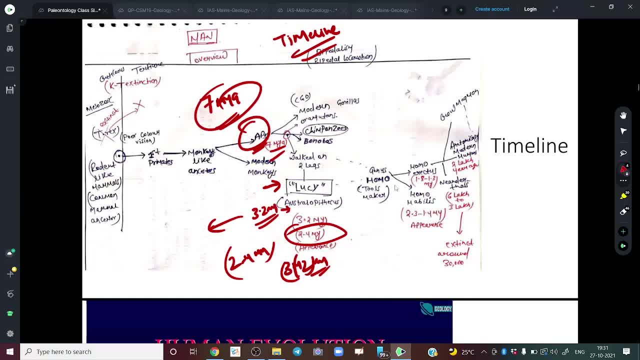 Which had bipedal locomotion. So somewhere around 2 million years. Right, This, Lucy, we are talking about 2 to 3 million years ago. Right, Then we have Homo habilis: It is somewhere around 1.5 million. 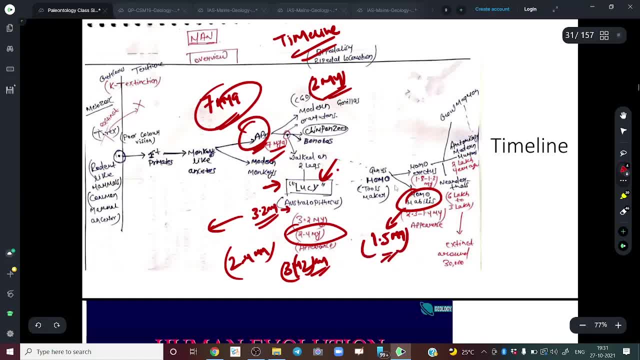 Right, This was 2 million, This is 1.5 million. Then we have Homo erectus, Somewhere smaller than 1.4.. So here, from various sources, I have written 1.8 to 1.3.. 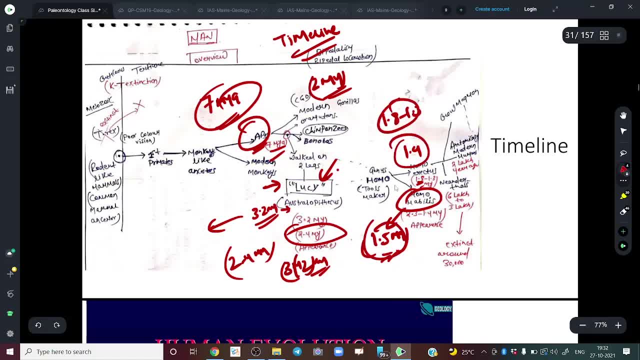 So just remember, it is 1.5. It is 1.4. Right. And from these Homo erectus evolved anatomically modern humans. So they are just like 0.2 million year old. So they first appeared just 2 lakh year ago on planet earth. Right. So we are. we modern human are very, very young vis-a-vis the history of earth Right. Earth history is like too much. It is 4.4600 million year old And we are just 0.2 million year. 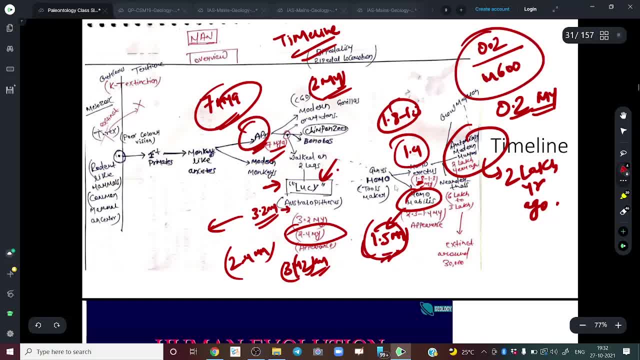 So we comprise. We comprise tiny, tiny part of earth's history: Right, The modern human, And similarly we have Neanderthals Right. They got extinct around 30,000 years ago And they appeared somewhere around 6 to 3 lakhs. 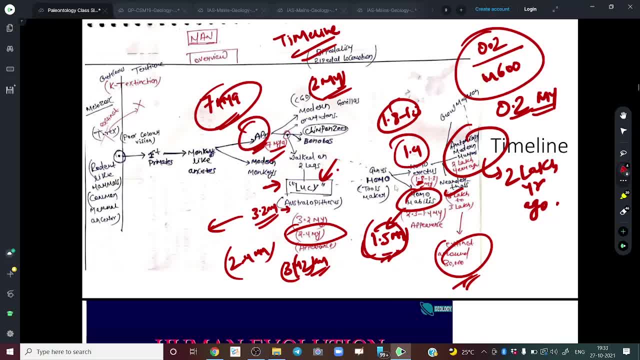 They appeared earlier than us, But they got extinct somewhere some 30,000 years ago, According to various theories, Right? So I hope you understand this. You should draw this diagram in your computer. You should draw this diagram in your copies. 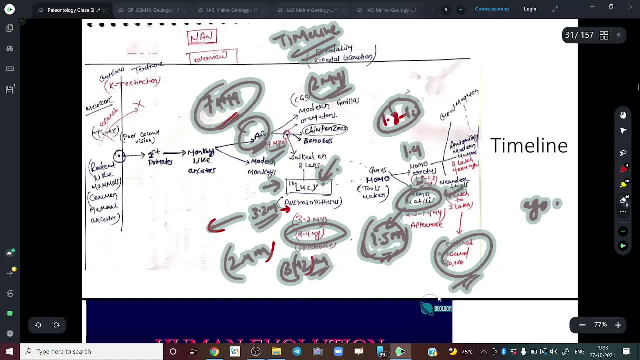 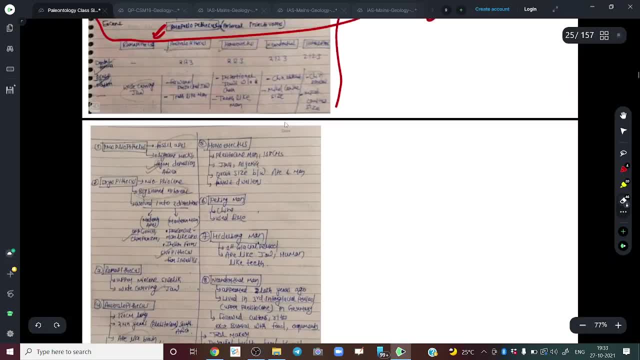 Copy for your overview And in exam. you can draw either this diagram or you can draw it in a vertical manner. So something like this Which we discussed Now. I hope this diagram would be more clearer to you. Wait, It will come again. 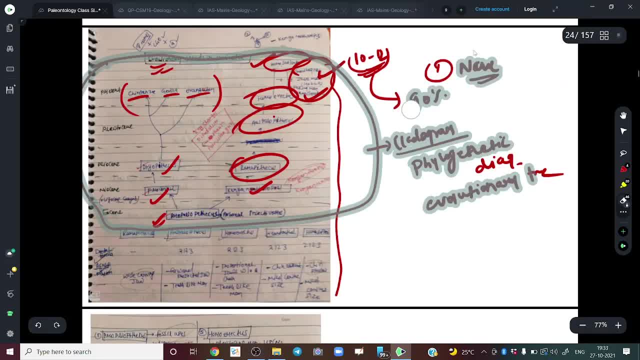 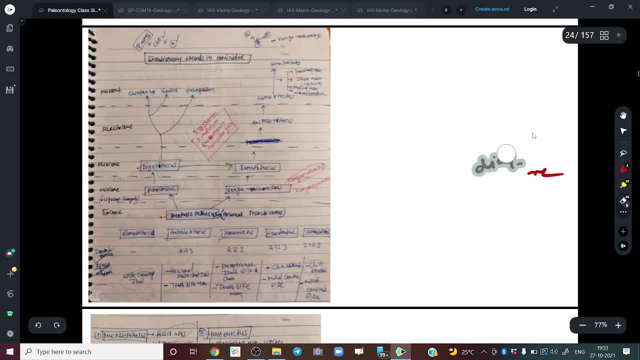 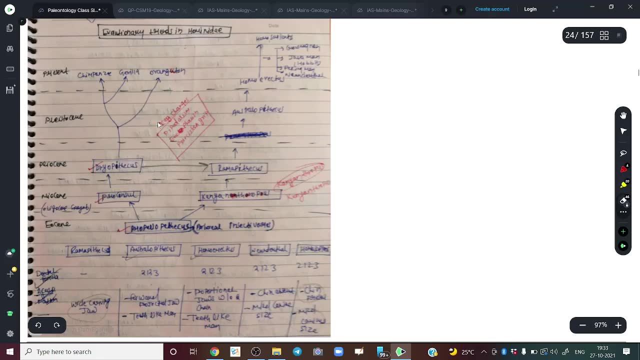 But I just want to tell you here The importance of this diagram is Here. you don't have to worry much about the timeline, See. So what I did is You are writing various species And how they are evolving, Right? 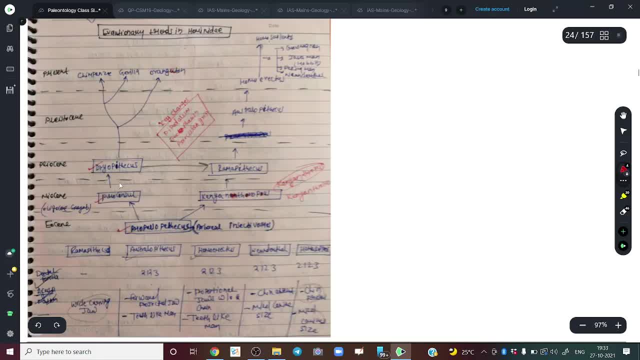 But you have also written this simple. If you remember the various epoch of Cenozoic time. You just write from Paleocene, Eocene- I think- Oligocene is missing somewhere- Myocene, Pliocene, Pleistocene- present. 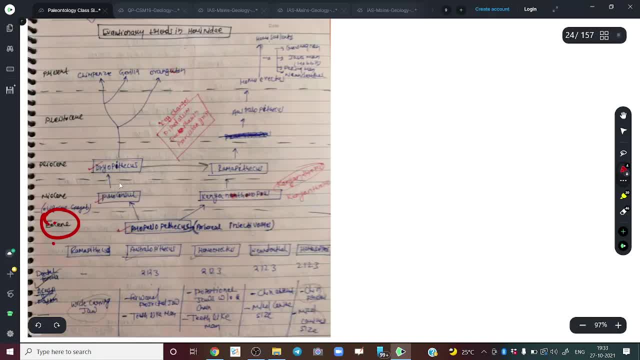 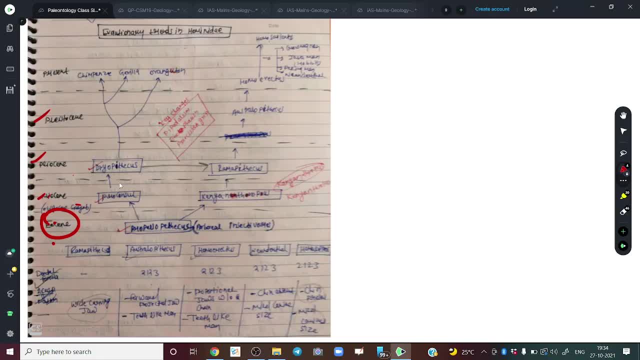 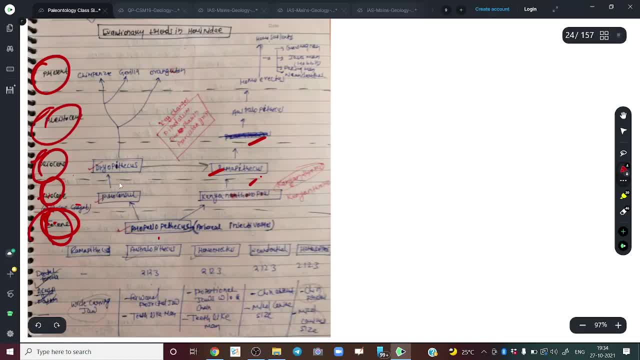 This may be, This may be. So it just simplified. It also gives a good timeline When this evolves And you just have to write something here, Right? You just have to write the name And then you can jot down something. 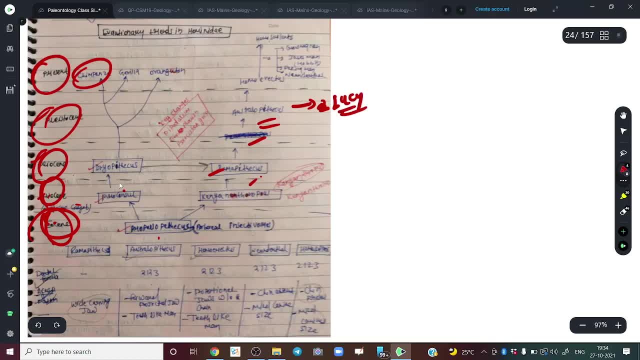 Like you know, Ocelopithecus- You can say The fossil Lucy- is an example of it. It was one of the first to develop bipedialism Like something like this: From home origin australopithecus, we have homo habilis, like it is missing in this diagram. homo habilis, then we have. 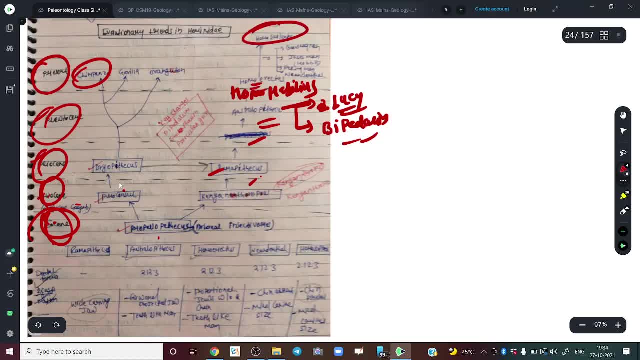 homo erectus. from homo erectus we have, we got homo sapiens. but then there were some five, six more cousins of ours which was present few thousand years ago but which got extinct, right, so that include chromaginon, zawa man. then we have, you know, peking man, we have neanderthals always. 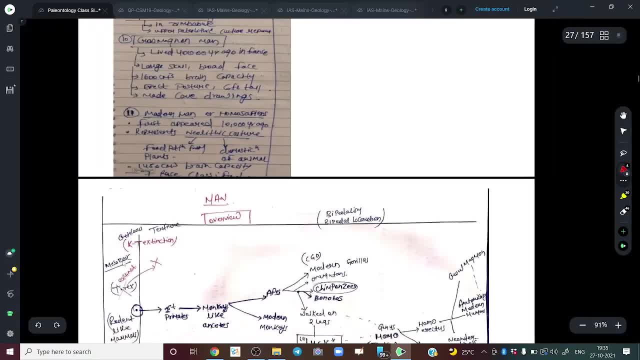 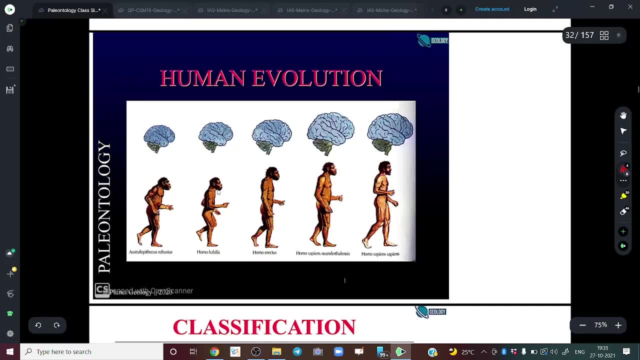 so we'll come back on this when we like, we'll have a detailed study of all this right and then we'll come back on it. so, like this is, this is a formal first slide, first lecture. till now, i just use my handwritten note- which were like, unfortunately, which are unfortunately in a 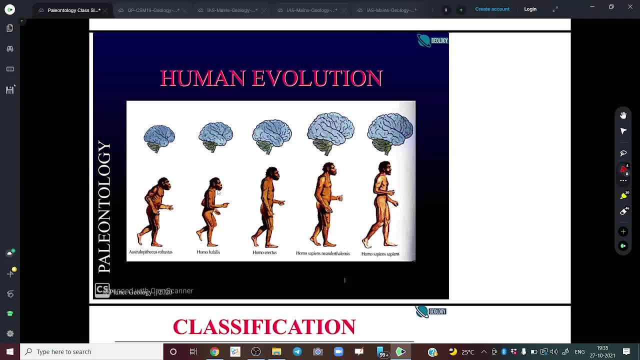 bad handwriting, but they were also very helpful. they will give you some idea about how you have to write an exam. so like just this. this is the first slide. this is just a random slide taken from google, so you also you first think and right in your copy what changes are happening right here. this is australopithecus, from australopithecus. 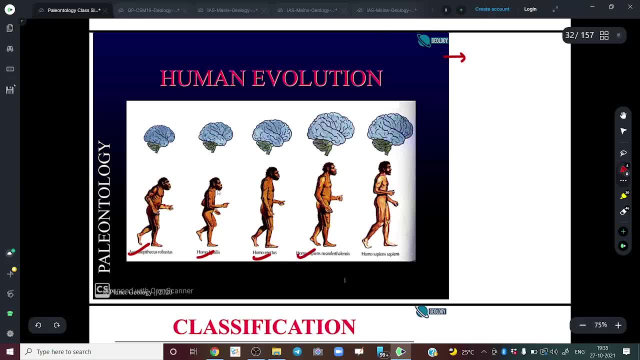 we get homo habilis, homo erectus, then homo sapiens, neanderthals, right, then homo. first thing, you should observe that evolution is not so simple, right? so, like here, it is written that australopithecus, we get homo habilis. from there, we get homo erectus. this is not the case, right, like we discussed here. 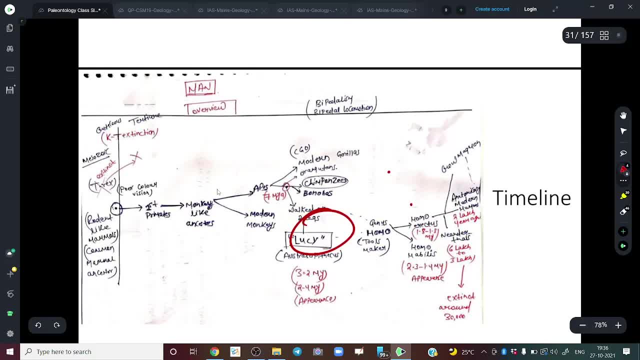 from australopithecus we get this homogenous from. one lineage goes to homo habilis and another goes to homo erectus, so it is not linear writing. it's like homo habilis to homo erectus, to homo sapiens. this is not the right. 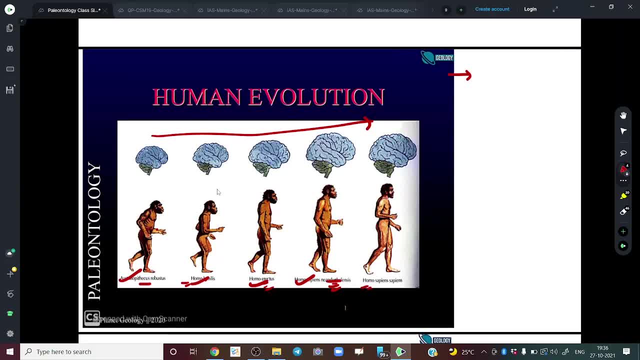 thing right, but this is just an introductory slide, so ignore this aspect, but know what what i mean to say. so like, just see what is the evolutionary trend. our topic is what changes are taking place, what is the evolutionary trend. so let's just see what is the evolutionary. 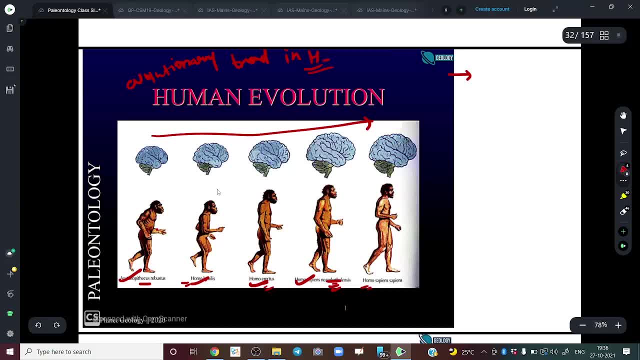 trend in humans. right, so these are different species, this is modern human. so what changes are happening? just see the picture and tell, tell, write in your copy. since this is a recording, recorded class, you cannot tell, so write this in your copy so like you can see what. firstly, this: 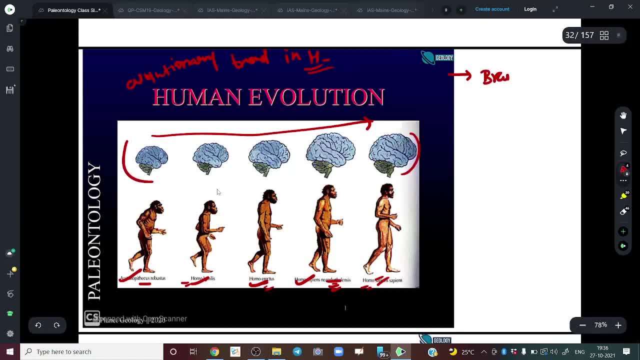 diagram is showing that the brain size is increasing generally. the brain size is increasing, right? you can also see that the bipedalism- all of them are bipedal, but you can say that this is one of the most erect species, like the posture is getting erect. the posture is getting erect with time, so this is one of 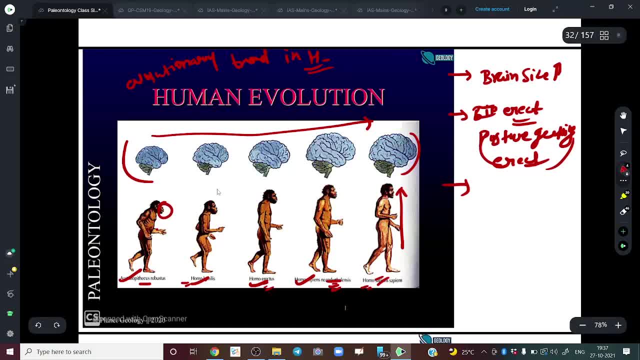 the changes right? you can also say that there is a change in the jaw, and here the jaw is more flatter. the jaw is getting flatter and in the earlier species they changed to the it is more protruded. what other changes? you can also say that the body hairs are decreasing. 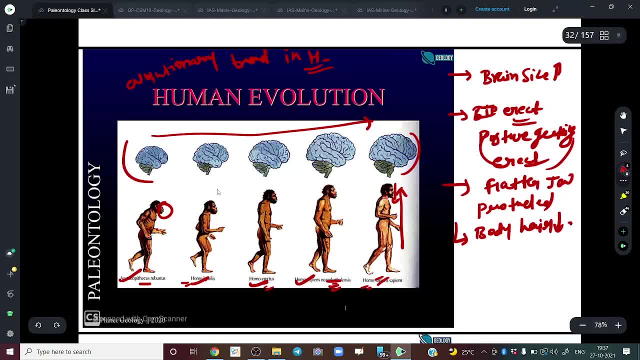 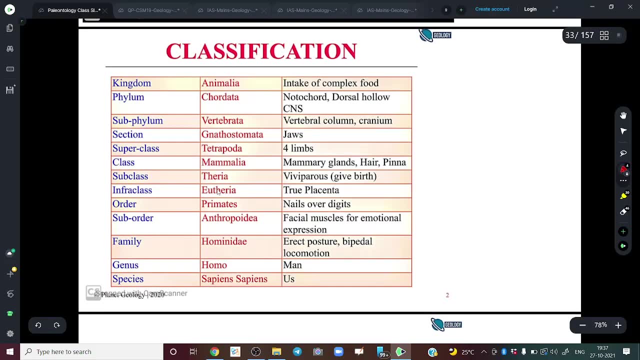 right? so, like these are some very basic, so this is what we are going to study. this is what we will be studying: what evolutionary changes are happening? what is the trend in various things? right? so, like again this this week we covered. this is just biological classification hierarchy. 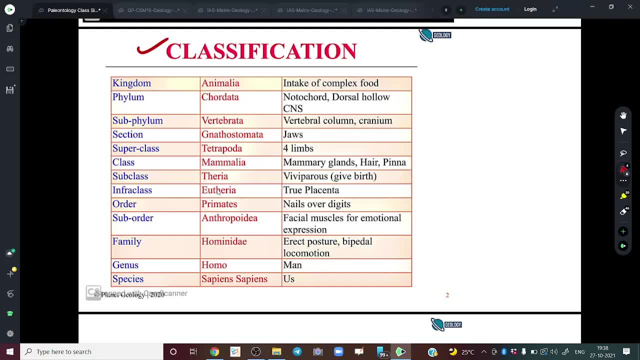 or the taxonomy, so you don't have to go in detail of all this, you can just remember we did it. the species is the homo sapiens, like it is about human. so you can remember this for man, elephant and horse, because these are mentioned in our syllabus. so we are. we are homogenous families, hominidae. 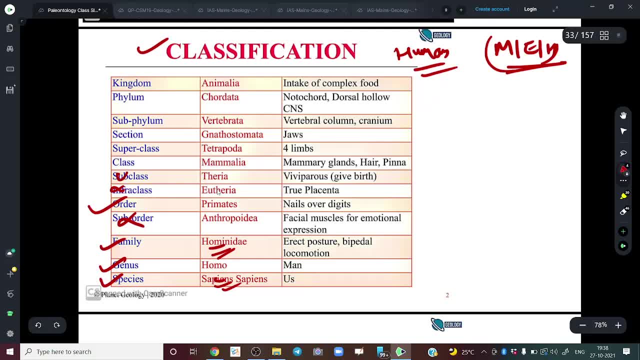 right, don't have to remember. suborder order is primate, homo sapiens hominidae and homo sapiens- hominidae. so we are homo sapiens, hominidae and hominidae. Class is Mammalia. right, ignore all this. Philem is Quadrata and Kingdom is Animalia. 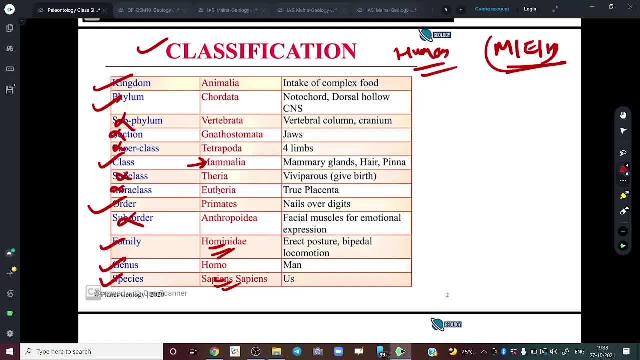 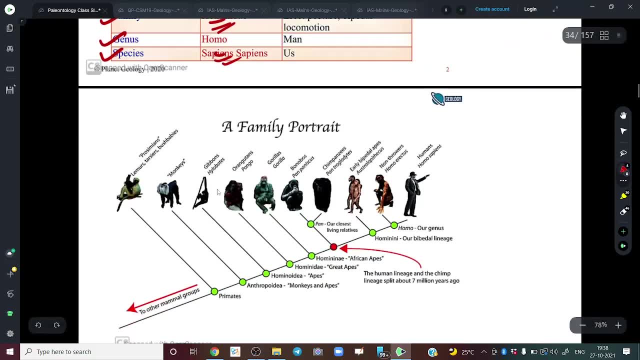 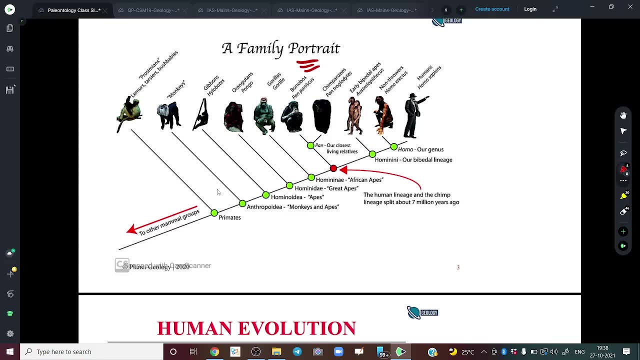 So this is something you can remember. maybe if you are writing an objective geology exam, then you might want to give a look at this column also, but this is not that important for our exam, right? So, like, this is again a family portrait. so again, like, evolution is not that easy evolution. 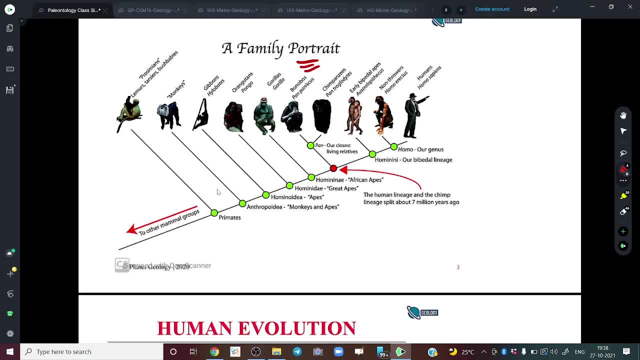 is not that straight forward or linear. it has a lot of web, a lot of linkages, so it is a very simplistic diagram. But just for your understanding, you can say that these were the earliest mammals. you can see, these are the mammals which are arboreal. 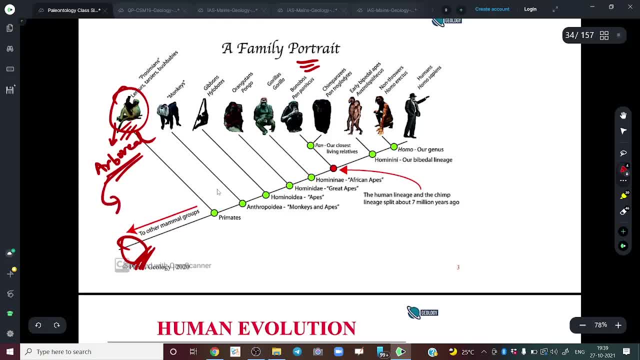 What is arboreal? Arboreal means the one which lives on tree right, which may live, which may eat some insect, may be some fruit, but it lives on tree. So from this you can see that this is a very simple diagram. 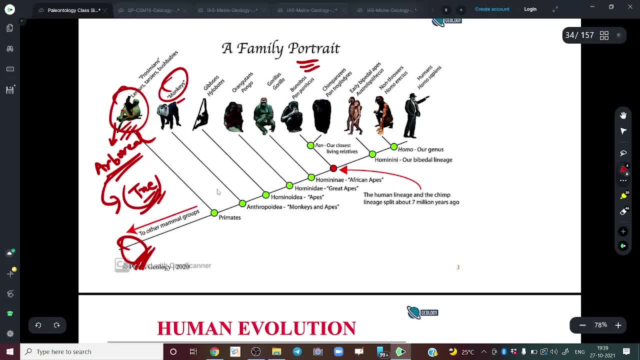 So from this you can see that this is a very simple diagram. So from this you can see that this is a very simple diagram. From this arboreal species we got this monkey-like ancestor, like we have gibbons. gibbons is one. 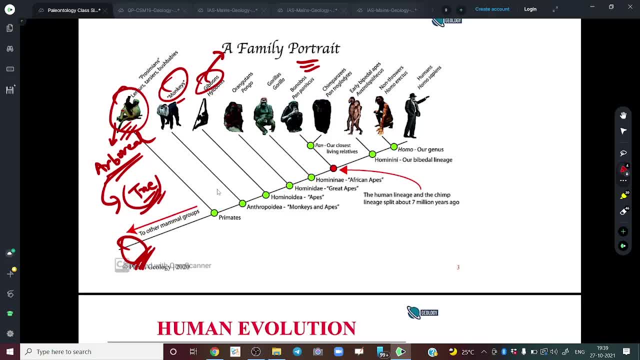 of the ape which is found in India. it is the only ape which is found in India. we have this orangutan, chimpanzees, gorillas. so this is bonobos. so this is what apes right. So from this primitive monkey, we have modern monkey and we have apes right. 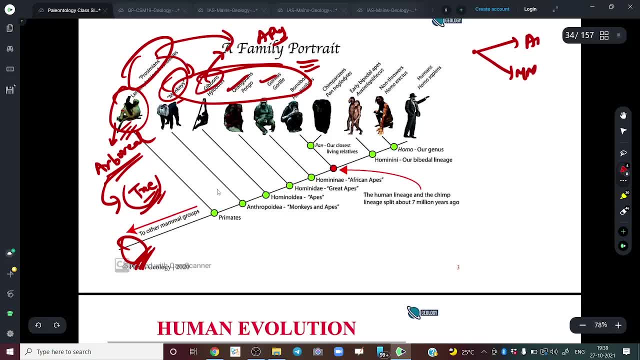 So these are two different branches: modern monkeys and apes from the primitive monkey-like species, From these apes, From these apes We have the aphids, We have the chimpanzees. also We have the earliest bipedal apes, which we call them Ostrelo Pythecurs. 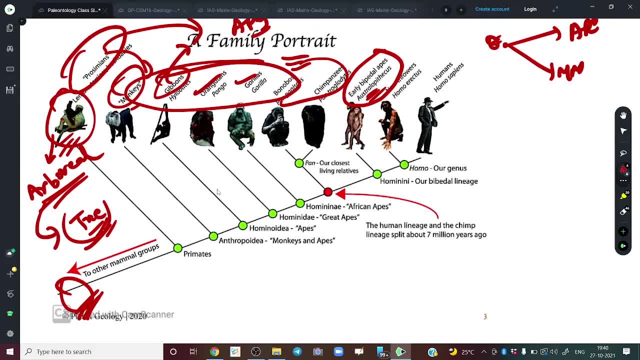 Like- I hope this slide is visible to you all- And from Ostrelo Pythecurs, we have Homo habilis, we have Homo erectus and we have modern humans, right. So this is a very simplistic way of understanding it, right. 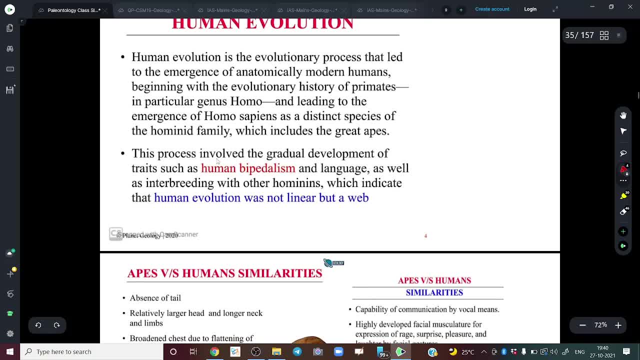 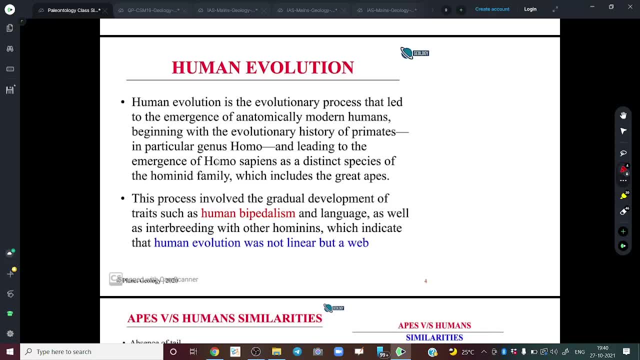 So, again, if you have to write an exam- and you have to- you have to define what is human, define human evolution in your own way, right? so what is human evolution? we in here, we talk about what we talk about. we talk about a evolutionary process that led to the emergence of anatomically 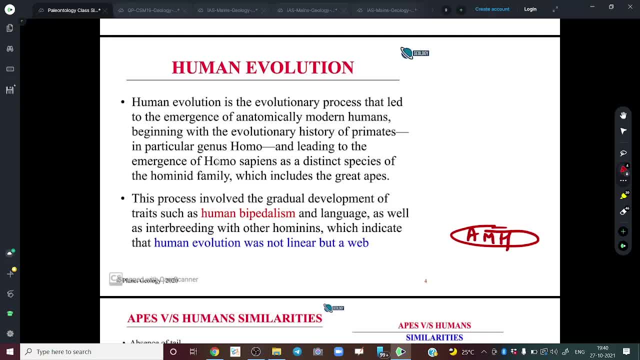 modern humans. from whom? from you know? from primates, right, this is human. evolution is evolutionary process that led to the emergence of anatomically modern humans, beginning the evolution with the history of primates, primates to from primates we get what from primates we get. 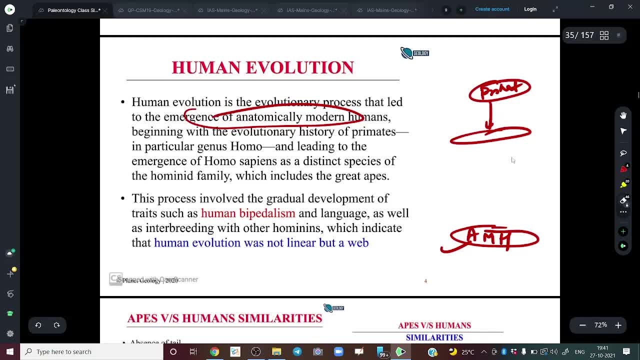 homo. the most important and most like the turning point in the evolution was the genus homo right, something like this, and from there we have, anatomically uh, modern man. and in this process there are various changes …. … like changes like bipedalism happened, changes in the cultural development, language developed. 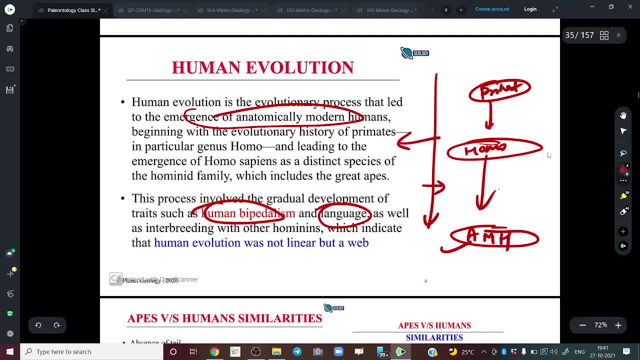 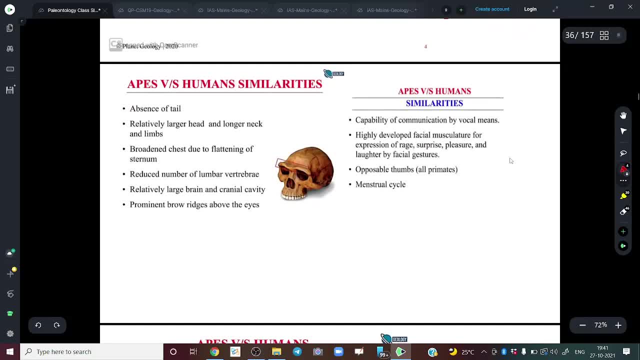 right, all these things developed. we started to, you know, control fire, we started to make tools, all these things right. so, uh, this is it. and then there are. there is a slide. i don't think upc is going to ask this: what are the similarities between apes and humans like? so we, we know what. 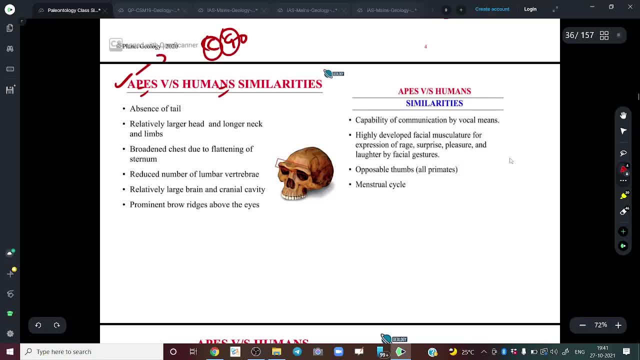 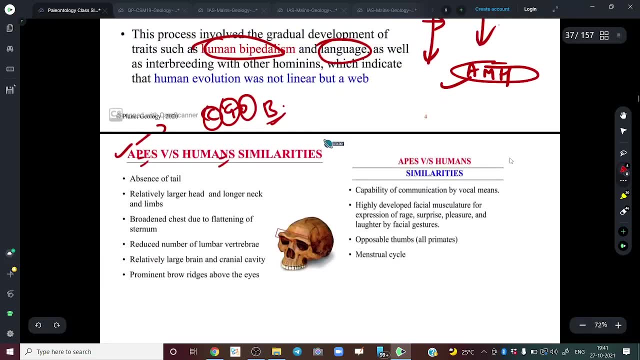 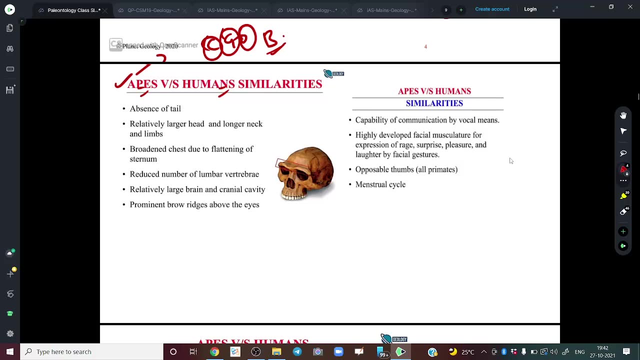 are apes. apes are c, g, o, chimpanzees, gorilla, orangutan, bonobos, all these things, the gibbons. so what are some similarities in them and what are some differences in them? this is just for your general understanding. this might not be directly asked in the exam, but still you can. 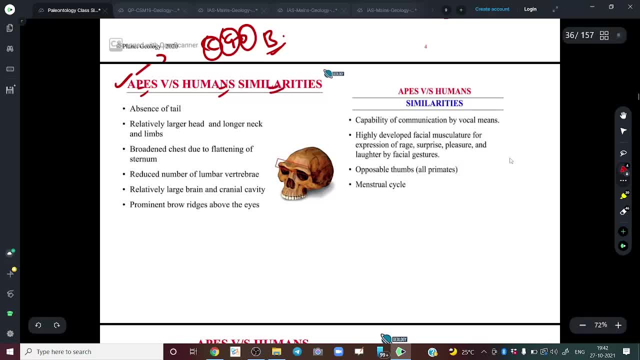 yourself make out, right? so what are the similarities? they both don't have tail, right? so monkeys have tails. so, like, losing tail is an evolutionary advantage, tail does have something to do with the tail, right? so what are the similarities between apes and humans? some its own advantage, but it does have some its disadvantages, like if, if you are in a fight. 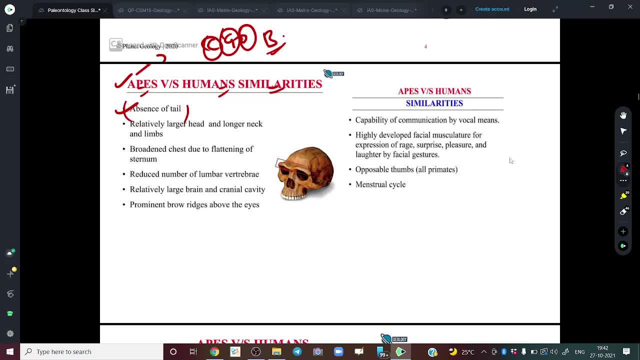 uh, this tail could be a weak point of yours, like it could be grabbed by your opponent from a distance and then you will be in trouble. so that is a evolutionary adaptation then. uh, the similarities is both have relatively harder, uh relatively larger neck and a relatively larger. 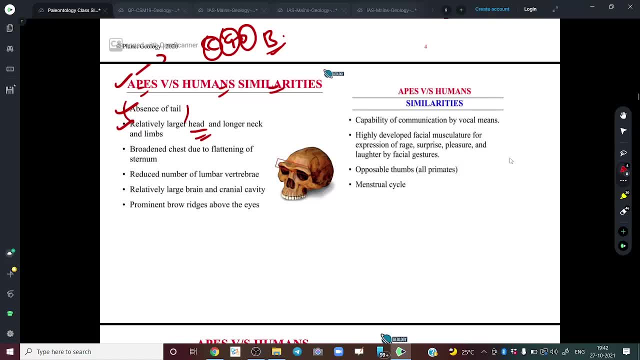 head. then, uh, there is this, uh, broadening the chest due to flattening of sternum. so sternum is basically the- uh, the outermost bone of your chest, something like this. then, you know, reducing the number of the uh, lumbar vertebrae, that is your backbone, right? 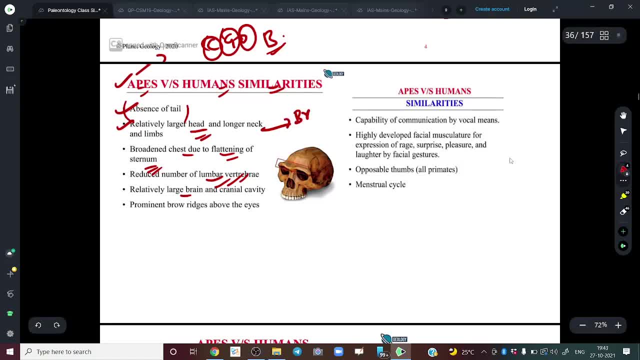 obviously brain size is increasing, relatively large brain size. so brain size in human is more than ape, but they won't have. they both have larger brain size than their ancestors, their primitive ancestors. and then this is this: they have prominent. both have prominent bro ridges above the eyes. you can see this diagram. both have this bro ridges right. so this, this is it. so this is more. 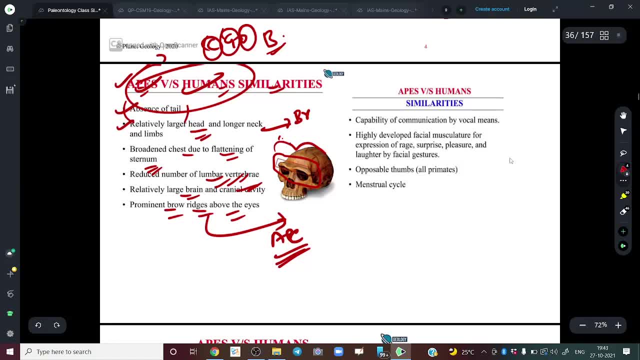 prominent in apes. this is more prominent in apes and less prominent than humans. right, since they have vocal means of communication. right, they have development of various muscles and, very important, both have opposable thumb. like what is opposable thumb that it is the ability of thumb to move in. 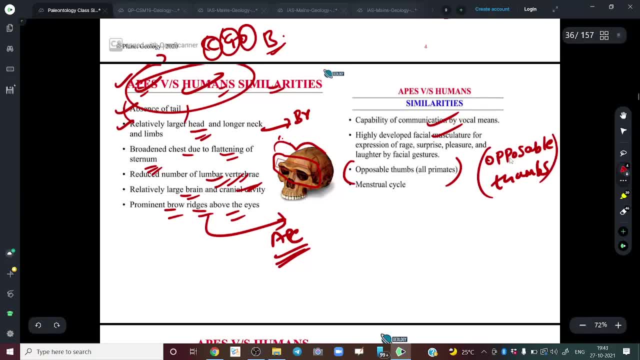 all the directions. so it is very important evolution point of view because it it helps you to use tools, it helps you to maneuver it, it helps you to grasp things right. so it is a very important and a very advantageous uh, very advantageous, uh, evolutionary uh, change, and then all the primates. 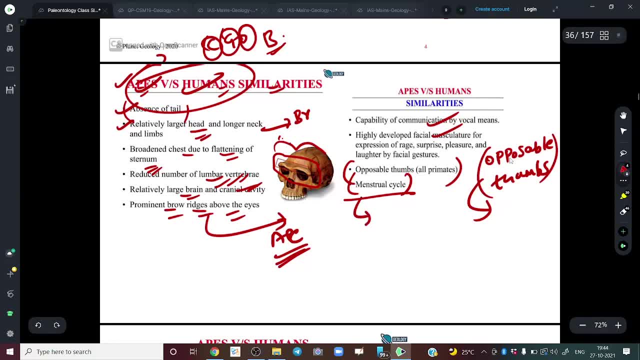 all the apes and all the uh humans. they have menstrual cycle right, so like in in other species. what, what is there in other species? uh, you must have a menstrual cycle right, so like in in other species. uh, you must have a menstrual cycle right, so like in in other species. uh, you must be aware that. 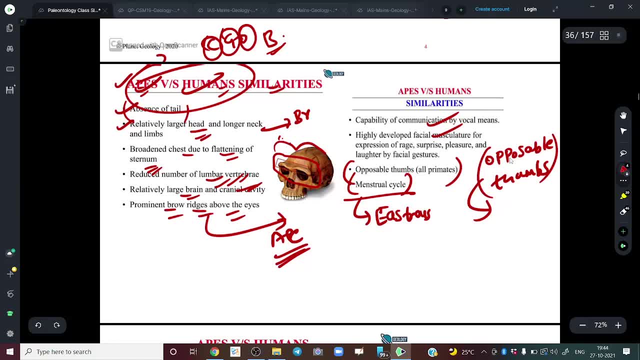 they have what we call as easter's cycle, right? so so what is the difference between these two like? in in menstrual cycle, the female is receptive for for almost all the time, so for throughout the year. but in this easter cycle it is not available throughout the year. it is available in certain. 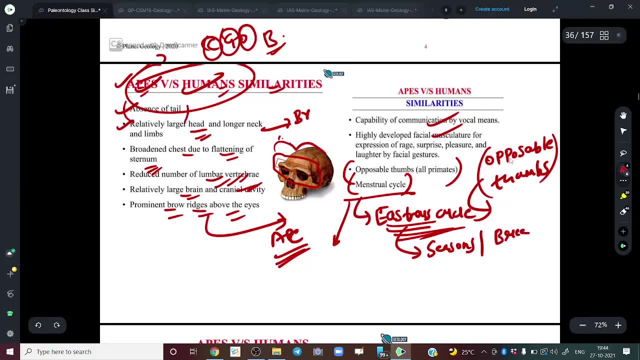 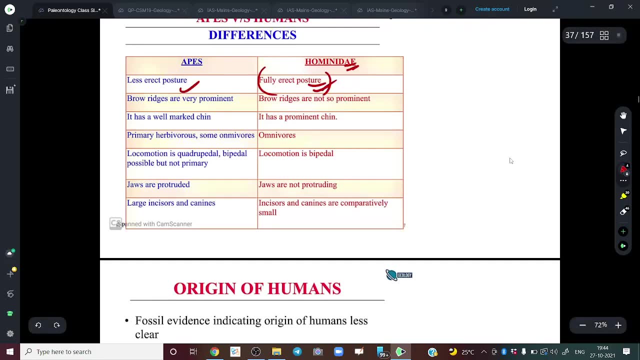 seasons. we call them breeding season. so this is the distinction between goosebugs and other hominids, right? so like this is a difference between these two, right? similarly, what are the differences? apes have less erect posture. humans have, you know, fully erect this. this woman and i have fully erect. 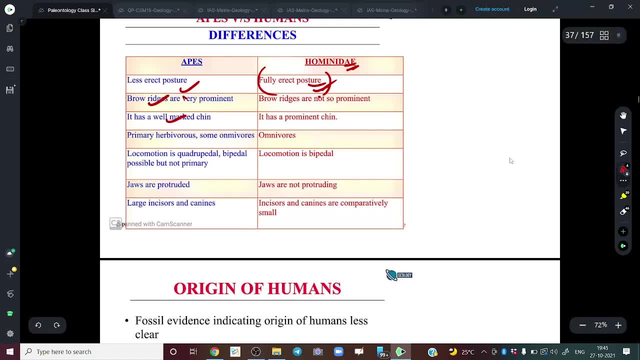 posture their bro Shawn stday's underől. just we just discussed. they are more prominent. these are not so prominent. like they still have a mocked chin. uh, ours is not. that marked the some of the beibellum, hominid and other ae supporter individuals. some of them are omnivorous. humans are mostly omnivorous, right? uh, that is the only difference in us, among cabeça humans and other hominid species are mostly omnivorous, right? these reappear them in amazing jeepster animals, as example we just just discussed. them are�온. 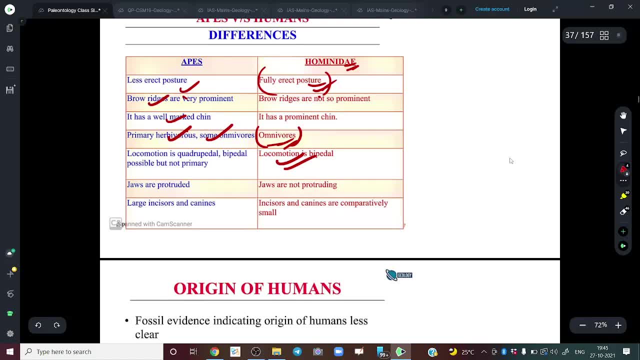 When the locomotion is bipedal. their locomotion is also bipedal but like their locomotion of AF is still quadruple Right. Like mostly, they use all the four limbs to walk. They can stand on two legs also. They can even walk on two legs, but that is generally not the primary mode of locomotion. 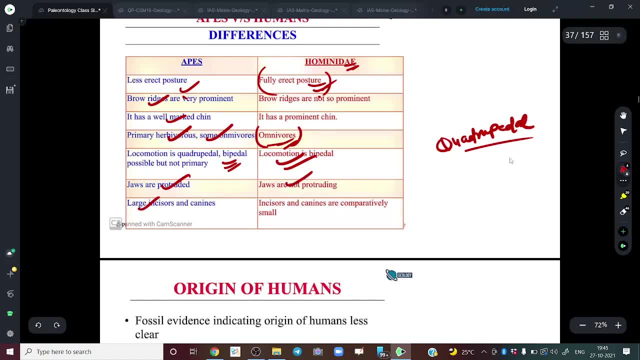 Right And jaws are protruded, not so protruded, They have large incisors and canines Like the dental structure is also different. So these incisors and canines, these are kind of teeth Like. so generally there are four kinds of teeth. 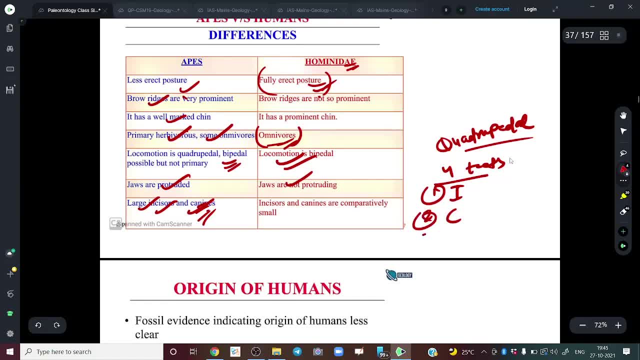 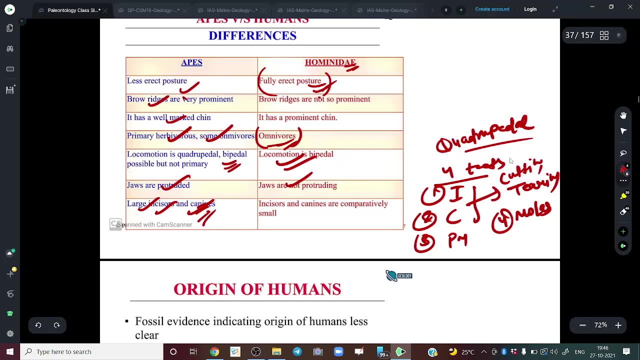 When we have incisor. second, we have canines. third, we have like what we have. we have premolars and we have molars. So these two are generally used for cutting and tearing And these are molars. these are generally used for what? 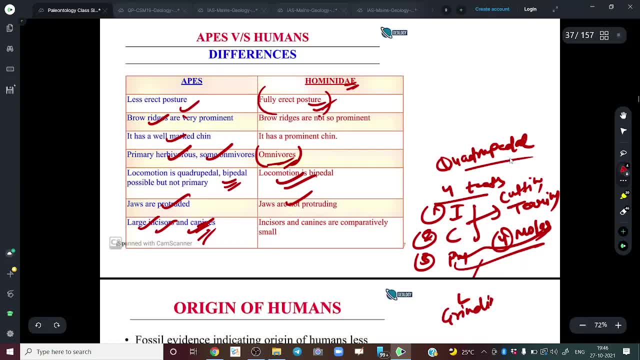 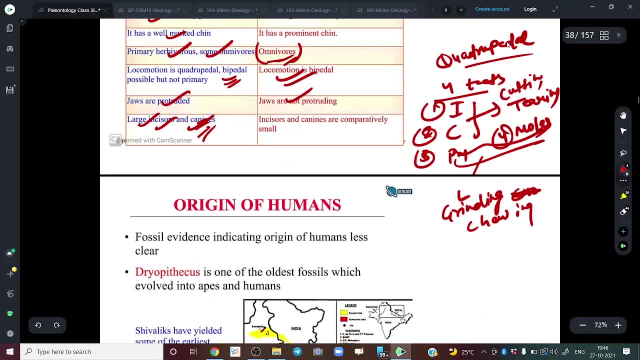 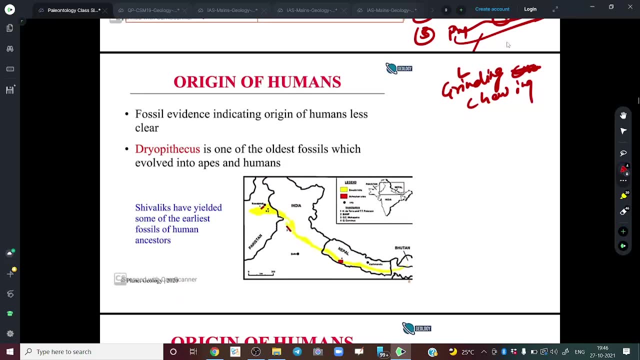 These are used for grinding, chewing, Right, That's it, And this is the last thing which we will cover in this part, That is, the origin of humans. So, like there were earlier, there was a theory that humans evolved. They first originated somewhere near this, in this Pakistan, India, Nepal and China region. 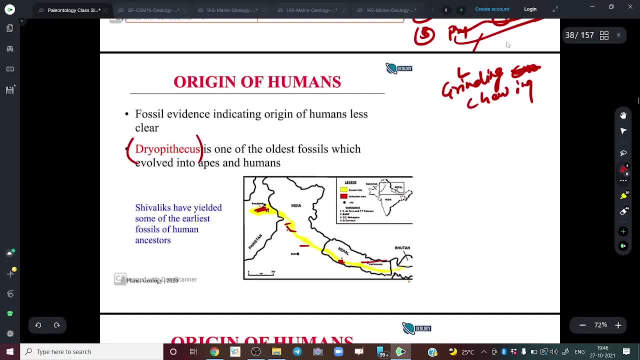 Right. So this Dryopithecus is one of the oldest fossils which evolved into apes and humans. Like you, just remember this name: Dryopithecus. It is one of the oldest. It is one of the oldest fossils. So even in the Shivalik, you all know what is Shivalik. 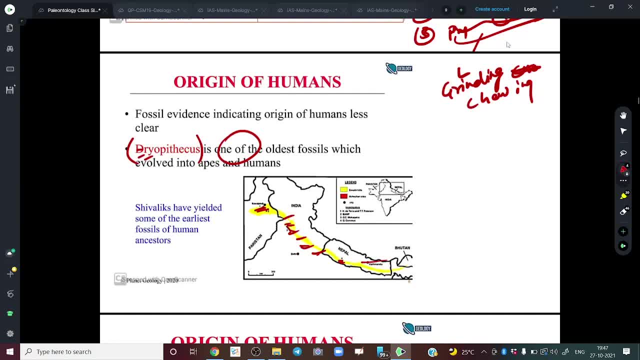 Shivalik is a part of the Himalayas mountain. It is the southernmost, southernmost range of the Himalayas, Like, not so great in height And most the younger one. So we'll study about it more in detail, about its paleontology, about its stratigraphy and its formation in stratigraphy. 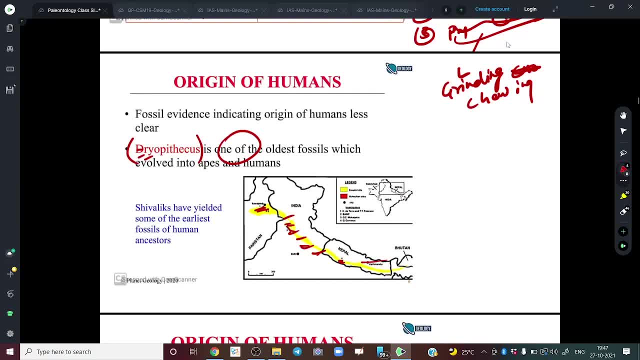 So this Shivalik, it is a heaven for vertebrate paleontology. So we have yielded a lot of earliest human fossil fossil of human ancestors in this area, Right. So like we have a fossil which we also discussed earlier, It is known as Ramapithecus. 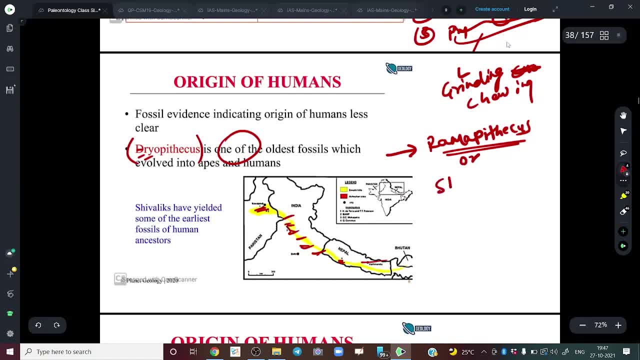 It is like some scholars call it Shiva Pithecus. They name it Shiva Pithecus And some scholars in their book they even write it as Brahmapithecus. It is more or less the same species, Right So earlier it was named as Ramapithecus. 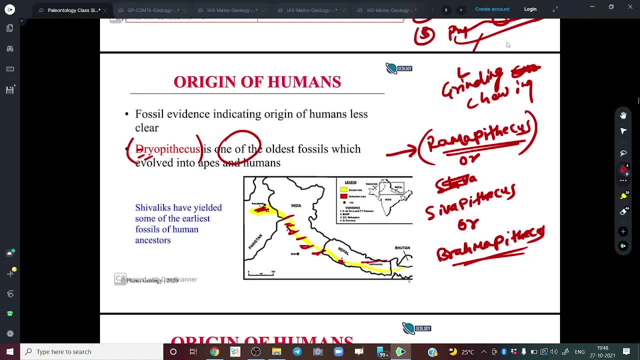 Maybe, like these are all are the names of the Indian gods, Right? So maybe the Lord Rama, Like the Ayodhya, is not much far away from the Shivaliks and also Lord Rama is also related to an army of, like a monkey army. 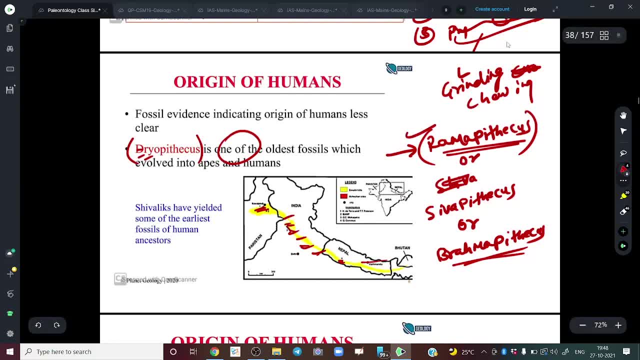 So in that way they named it Ramapithecus and then they named Shiva Pithecus, Shiva from the Shivalik mountains Right. So this is also one of the earliest fossil. So there were speculation that human India or the region near India 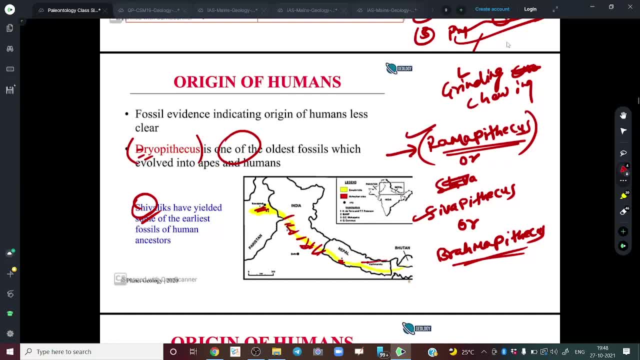 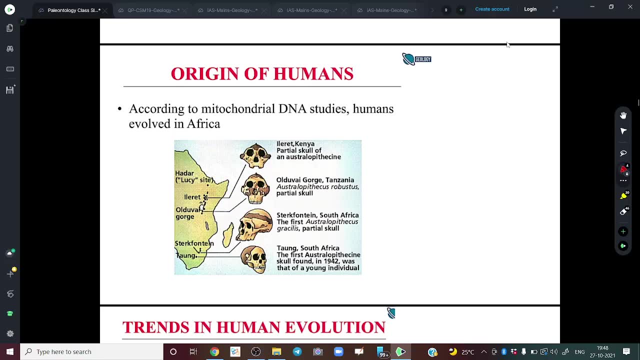 These are the cradle of human civilization And from here the first human species. you know it is. it appeared in, it, evolved Right. So this was one of the earlier theories. like what the decent, the most modern theory, they conclusively says that the modern, or the present human, they first appeared and they evolved in the Africa, somewhere around this area. 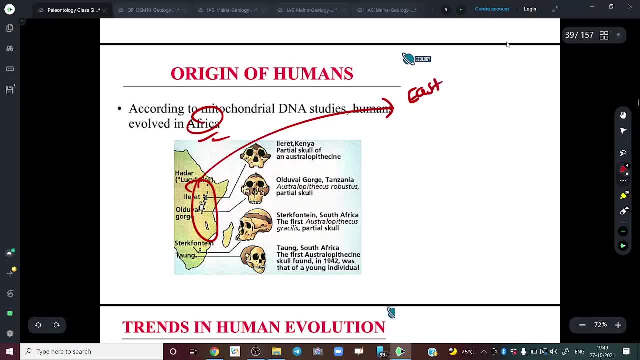 This is what this is: the East African rift. in East African rift right, or it is also known as famously known as Afar region, the modern Ethiopia right, we have a lot of like. we discussed about australopithecine. then we have some other species. they were found in some other fossil. they were found in Tanzania, South Africa and further till. even this, this part. 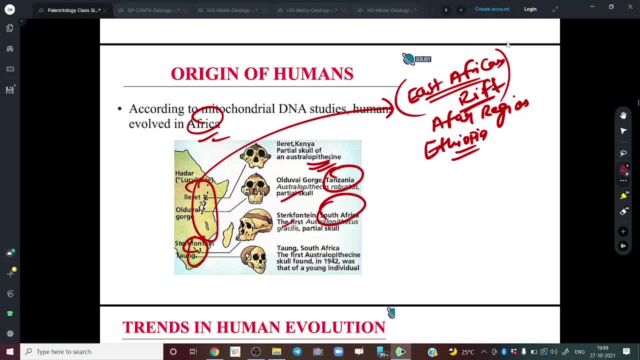 So now, According to the mitochondrial DNA studies, humans evolved in Africa, Right, So this is more or less conclusive, but there are still a lot of debates, a lot of research going on on all the things. But as a geology student, we don't have to go in all those details. 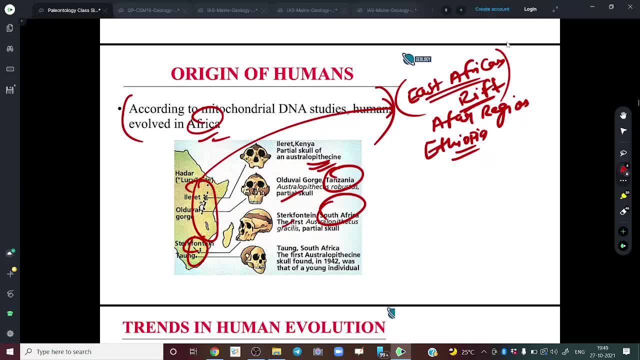 We need to maximize our marks Right. We need to like: there will be 20 or 25 market question on this. We just need to ensure that we score 80 to 90 percent in there. for that We need to write maximum keyword, maximum information. 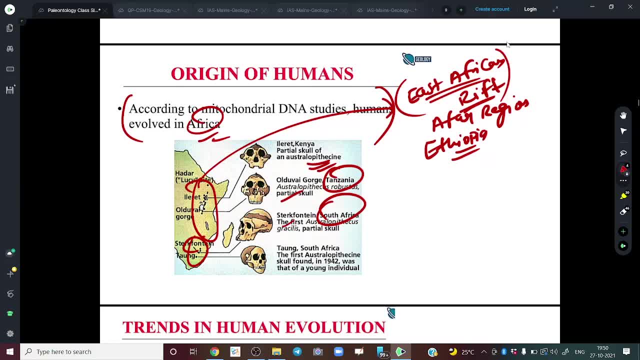 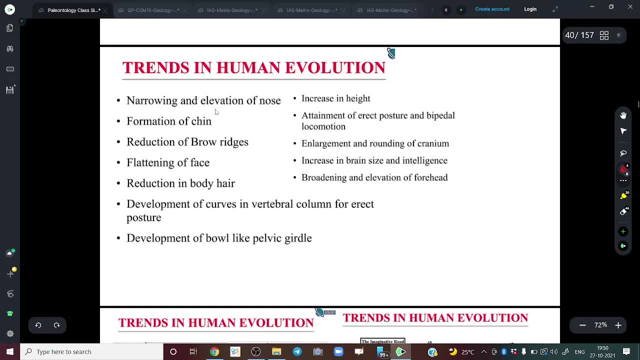 And we should try that We should avoid unnecessary controversies. So like this is a accepted viewpoint, Right? So this is it. And then one more thing. just like we discussed in the first, first picture, the trends in human civilization, the same thing is summarized here in this slide. 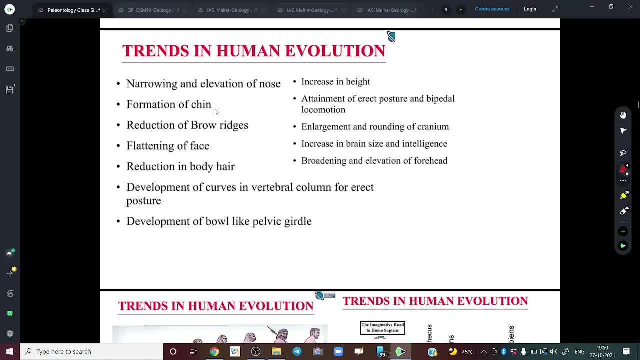 Right. So like what are the trends in human evolution? Like we discussed, there is an increase in the height. There is attainment of the erect posture- Very important- bipedal locomotion is happening Right. With time, brain size is increasing. 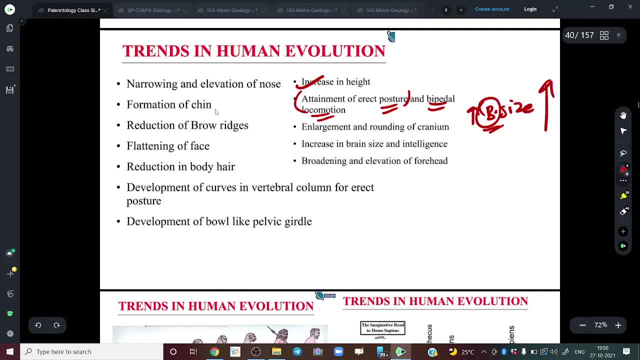 Like this is: brain size is increasing with time, like also intelligence is increasing. then there is broadening and elevation of forehead, reduction in body language, reduction in body here Right. Then we have this narrowing and elevation of nose, formation of chin, reduction of brow ridges, all these things like we have discussed. similarly, development of bowel like pelvic. 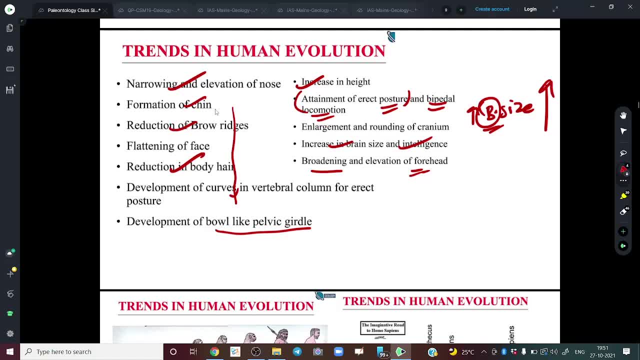 So like this, this is a primal really related to holding of the pregnancy Right. So these are all evolutionary Change, the trends happening in the human evolution, So you could write this in exam. So if somebody is asking this question, always draw the diagram that is discussed in the first slide: the human evolution with phylogenetic diagrams. After that scrubs something on that diagram. And if it is a 286, then match those 3 with theirAbs approximately. Yeah, So like there is an overnight pendulum where man is實nelCO2 present, but it is not this, and there is power symbolization. Now the surface here is a Erpin just because people referring this or on this perspective during digital consumption. So where this is a нейligic rural private model, 반 aston, tiny scale work, really clearn. Learn know about funds currently, but bring some information. 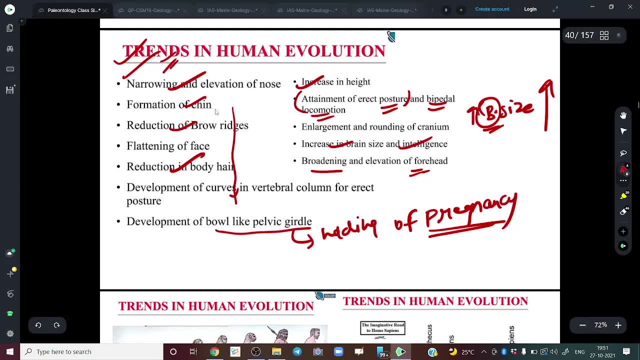 If I marker, write all these points. What are the trends in human evolution? These are all the trends happening. Maybe, if you have some data about brain size, write that data That we will cover in the next class. Similarly, this is what is happening. 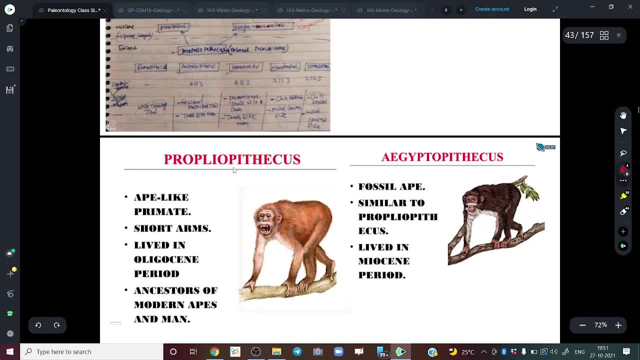 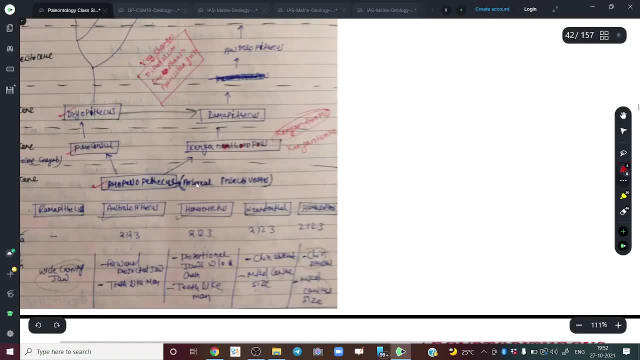 So I think we will stop it here. From the next class we will study this diagram in detail. What we will do is we will pick up each species. We will pick up proper Iopithecus And we will discuss what are its characteristics. 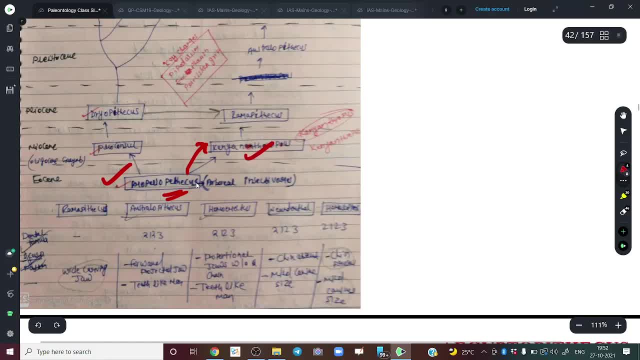 And then how changes happened And it formed into Cananthropus or Proconsul, Something like that. How then we got Diopithecus? Like we discussed? it is one of the oldest fossil to be discovered, So what are its features? 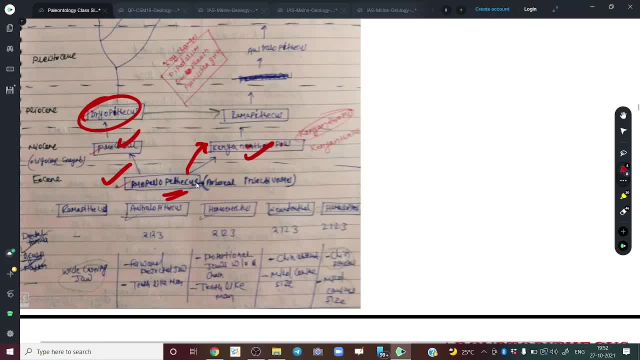 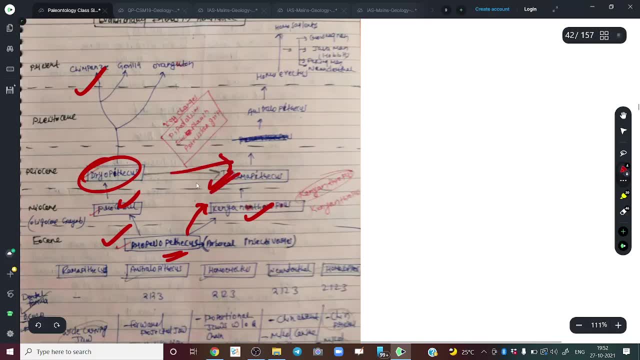 How it looked like And how it evolved into this modern ape, And when lineage went to this Ramapithecus which is found in Shivalik. Then about Lucy Right And the Australopithecus species Homo erectus, Homo habilis, Homo sapiens. 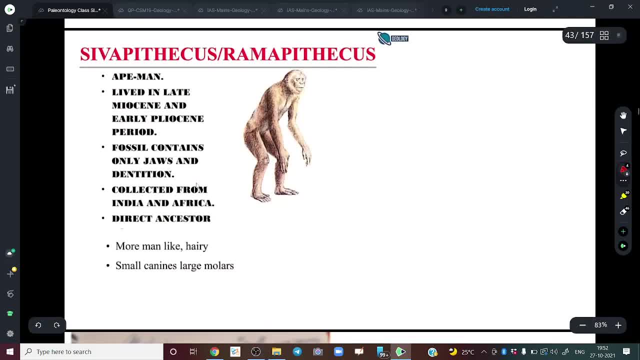 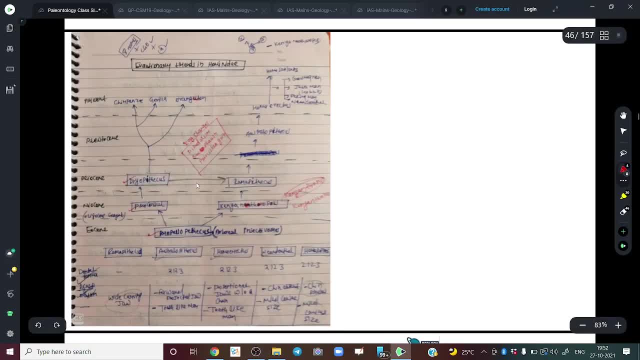 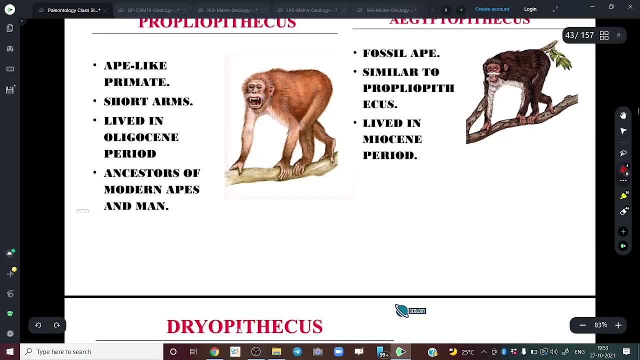 So from next class we will pick up very briefly something about them. We will also talk about brain capacity and all these things, Advantage of bipedalism, all these things. So this is it. So I think we'll end the class here today. 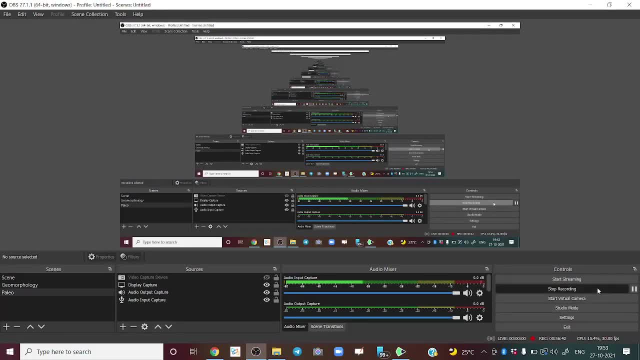 And then we'll have next session tomorrow. Thank you.